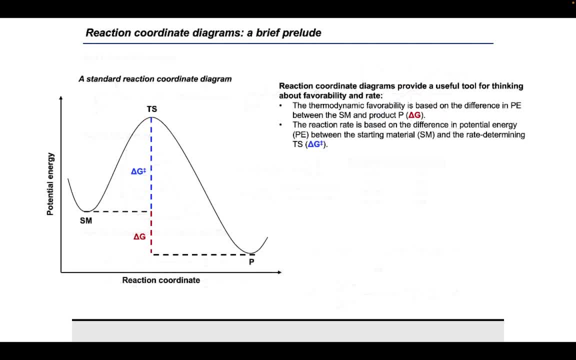 these often intimidating experiments. Before I dive into these topics, I first want to introduce the reaction coordinate diagram. This graph allows us to track the energetic favorability of the different ground states and transition states as the reaction proceeds On the x-axis. is the reaction coordinate? As the reaction proceeds, we move from left. 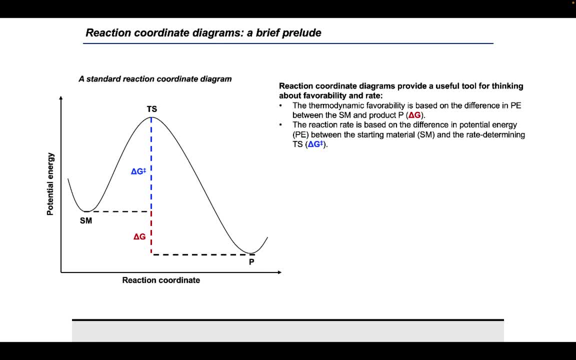 to right on this graph On the y-axis is potential energy, which describes the stability, favorability or statistical likelihood of the different chemical states of the reaction. Now, in this case that I have shown here, we have a simple one-step reaction where the starting 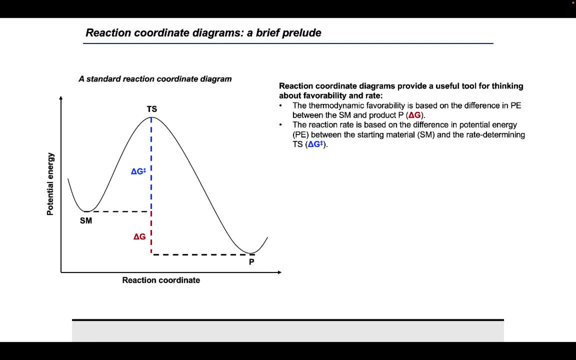 material goes to the product via a transition state. Delta G double dagger, shown here in blue, describes the amount of energy required in order to convert the starting material to the product, which is correlated with reaction rate. Delta G in red is the difference in. 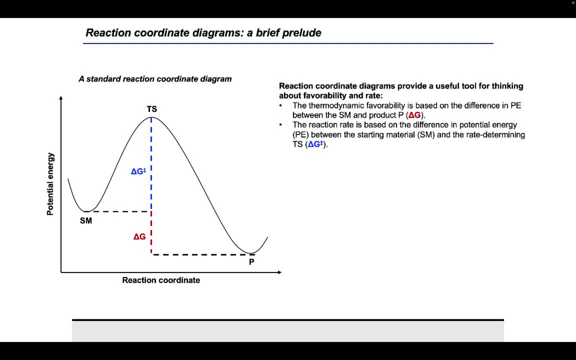 potential energy between the starting material and the product, which describes how favorable this reaction is – ie in which direction the equilibrium lies. Now, the main question were going to ask today is: how does changing the nature of our substrate change? delta G and Fosten microwave. 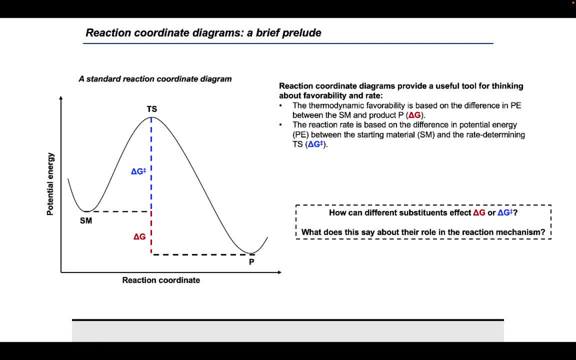 I think it can be broadly understood from Fosten sake, but it is quite pairly and equally important. This means that in the case of any material snobs, energy will not change the more of a focus. delta, G, double dagger. All right, moving into part one, Hamet analysis. First we're 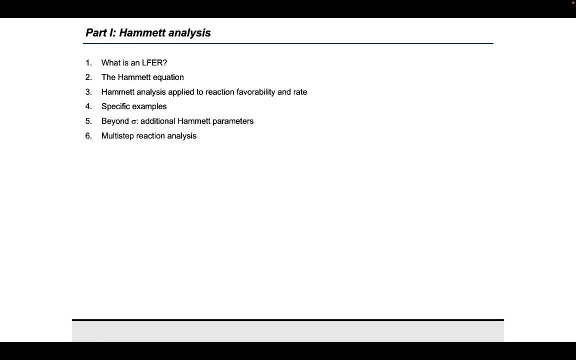 going to discuss what linear free energy relationships are, which then leads us into the OG Hamet equation. We'll then use this Hamet equation to understand substituent effects on reaction equilibria and rate. Next, we'll return to expand our understanding of Hamet parameters. 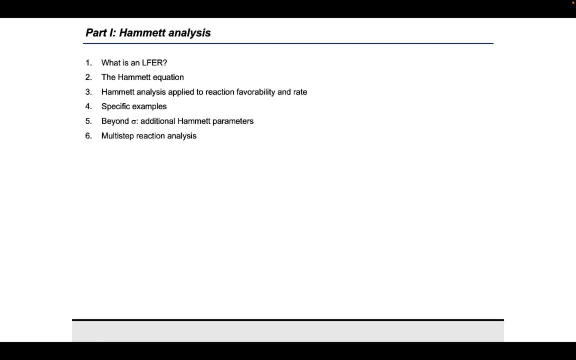 and then look at some more complex examples. Buckle up Linear free energy relationships, or LFERs, empower us to understand why substituents might affect the rate of a reaction. In order to do this, we draw a relationship between substituent effects on a simple 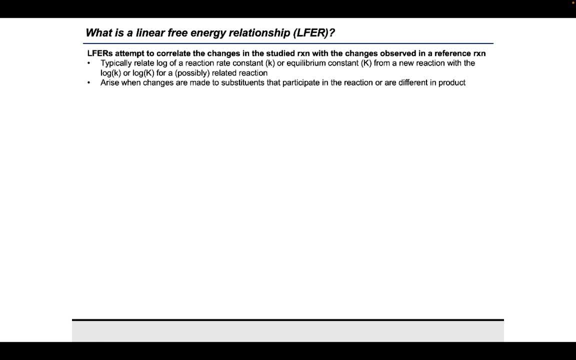 very well understood- reference reaction and then the substituent effects in our reaction of interest. So once we have measured the change in rate for change in substituents for our reaction of interest, we can now draw a relationship between substituent effects on a simple, very well understood 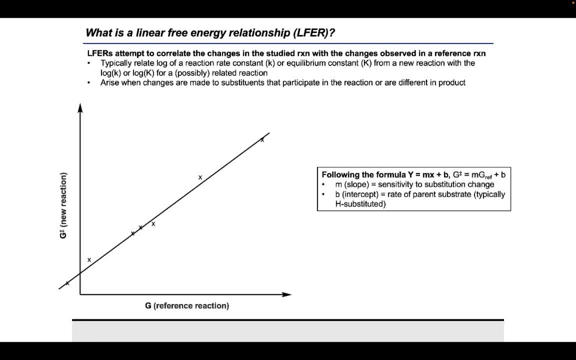 interest. We can then compare how those same substituents affect the rate in the reference reaction. A linear correlation between the two then tells us that the effects are proportional, and then the magnitude of the slope tells us the degree of similarity between the two reactions. 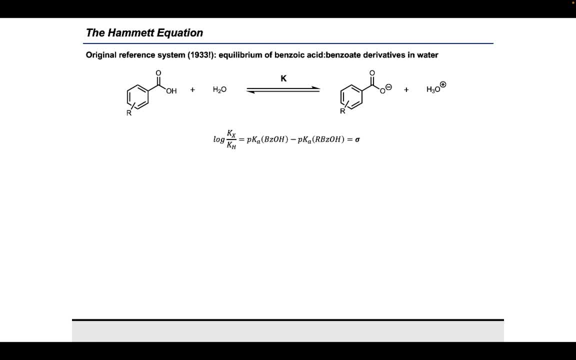 The concept of LFERs was first introduced in the early 20th century and it's been extensively used for the past 80 years. There are several different LFERs. The Hamet relationship is by far the most commonly used and can be used to study electronic effects. The Bronsted LFER is used. 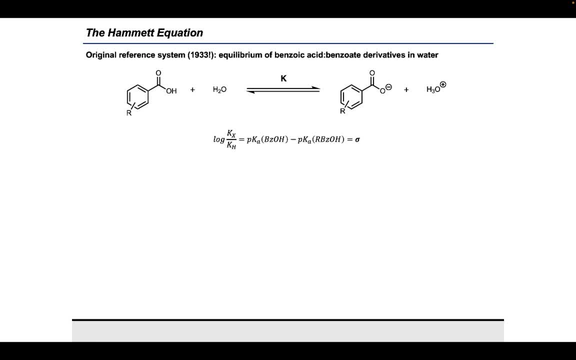 to study acid-based catalysis, particularly in the context of enzyme kinetics. LFERs to understand steric parameters are more complicated and the Taft, Charton and Steramol parameters all attempt to model the steric effect of substituents Shown here. the Hamet relationship uses the deprotonation. 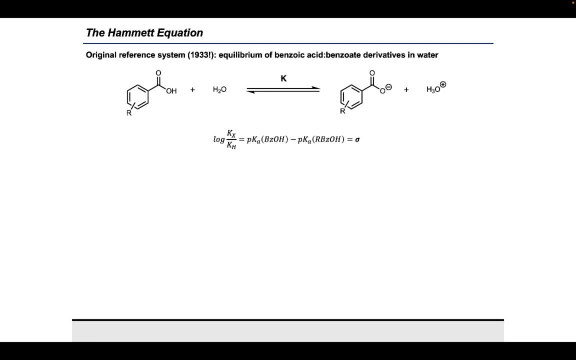 of benzoic acid as the reference reaction. The equilibrium for this deprotonation is affected by the inductive and field effects of the substituent, but not by resonance, because the negative charge on the benzoate cannot be resonance delocalized into the aromatic ring. Measuring the pKa's of a series of acids gives: 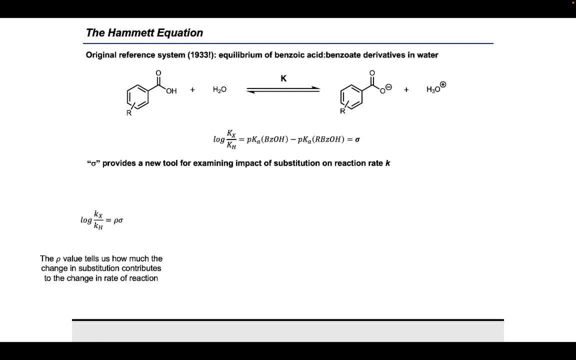 us the sigma value, which is the difference in pKa's of different benzoic acids. The sigma value can also be represented as the log of the ratio of the equilibrium constants. Note that all LFERs typically use log 10.. This is an artifact of having used pKa's which are always base 10.. 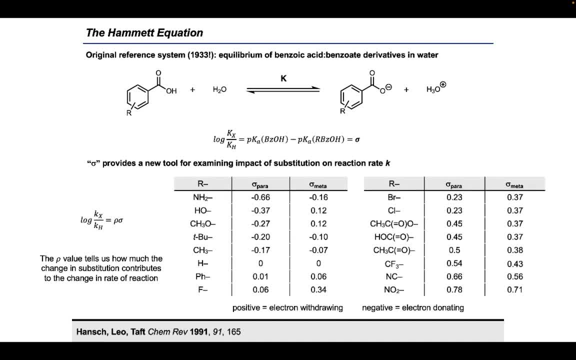 Lots of sigma values are known. pKa's are measured in water, The unsubstituted with H is zero by definition. and then substituents that are electron wet drawing have a positive sigma because they stabilize negative charge And thus increase the equilibrium constant for the deprotonation of benzoic acid. 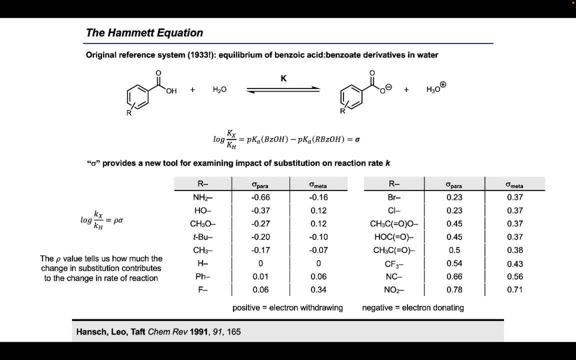 Substituents that are electron donating have a negative sigma value because they destabilize negative charge and thus lower the equilibrium constant for the deprotonation. In looking at this chart, we also note that there are different values for the same substituent depending on: 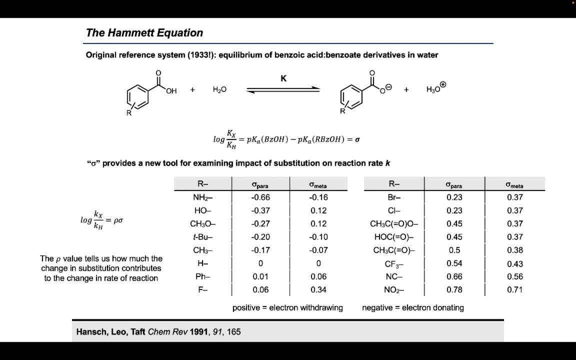 whether it is in the meta or para position. These values are typically not used for ortho substituents because at the ortho position, the steric effects of the substituents become much more important. When comparing the meta and para values, some of them are really different, For example, 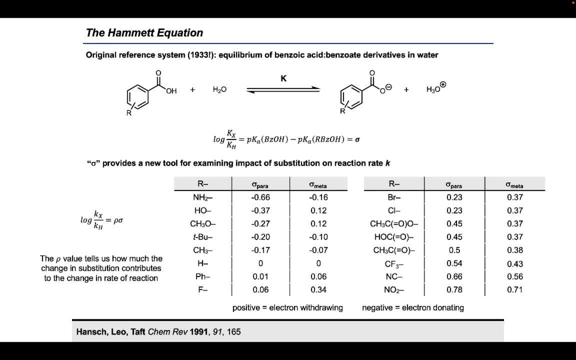 alkoxy substituents are electron donating when in the para position, because they can draw resonance structures that place negative charge on the ipsocarbon, which destabilize the benzoate, while they are actually electron wet drawing in the meta position purely because of their inductive effects. The same is true for amino substituents. Now, when looking at new 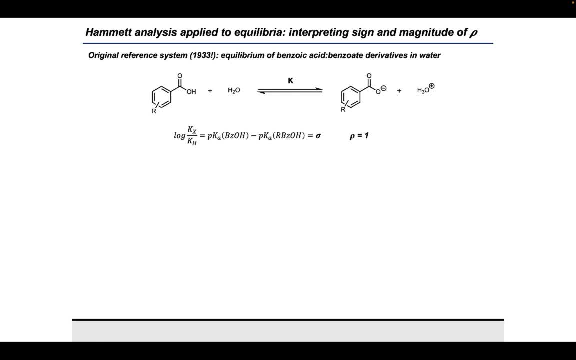 reactions. we have an equation that allows us to relate the long change of the equilibrium or rate change of two substrates in the new reaction to the reported sigma values. The equation is shown here. In this case, the rho value defines the sensitivity and direction of the reaction. 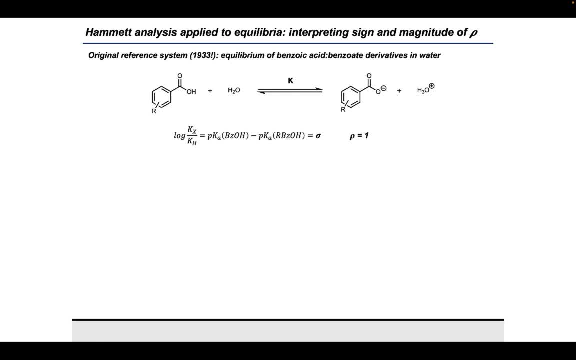 equilibrium or rate change caused by substituent change relative to the effects observed in the deprotonation of benzoic acid. If the rho is positive, that's indicative of the reaction having similar features, and so maybe there is build up of negative charge as well. If the rho is. 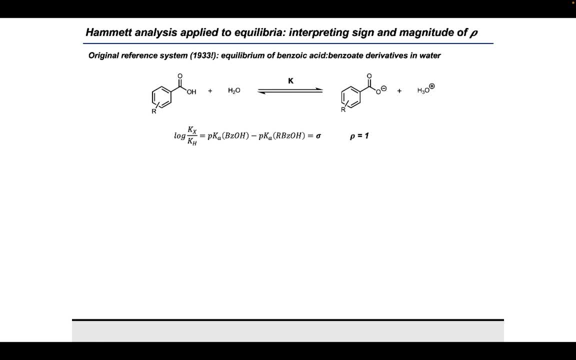 negative. that means that the effects are opposing, likely due to build up of positive charge going from the starting material to product. Let's look at a few examples We have here. first the deprotonation of substituted phenols. Here the molecule develops negative charge in moving from 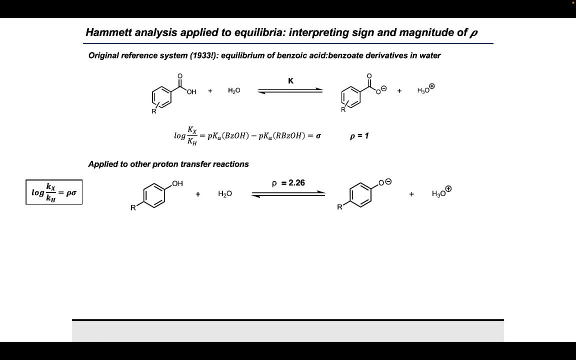 the starting material to the product. hence the rho is positive. The negative charge is now directly adjacent to the ring, one bond shorter than in benzoic acid, And so because of this the substituents exert a greater influence on this reaction, and thus the rho is also much. 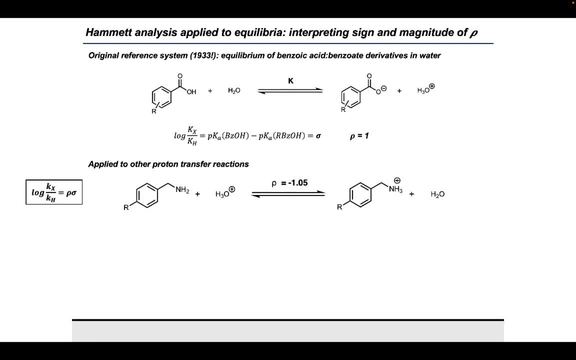 greater than one. In example two we have the protonation of substituted amines. The molecule develops positive charge in moving from starting material to product, so hence the rho is negative. The positive charge is approximately at the same distance, in terms of bonds, from the substituents. 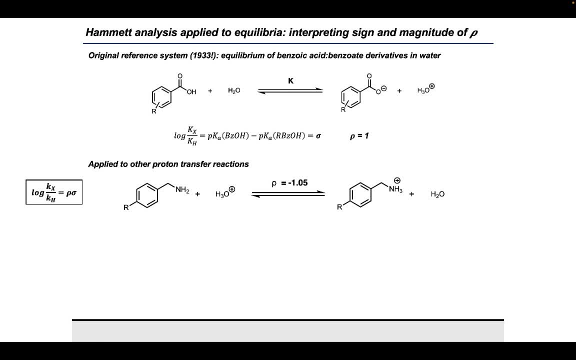 as the negative charge in benzoic acid. hence the absolute value is similar and the rho is around negative one. In example three we have the protonation of substituted anilines. Here the molecule develops positive charge in moving from starting material to product. hence the rho is 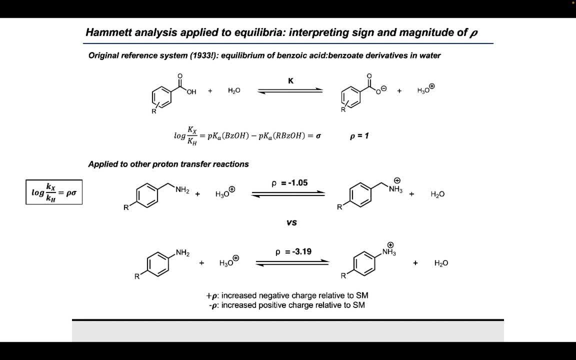 negative. This time the positive charge is closer to the substituent by one bond as compared to benzoic acid and, as a result, the substituents affect this equilibrium much more than they affect benzoic acid, and the rho is much more negative than just negative one. 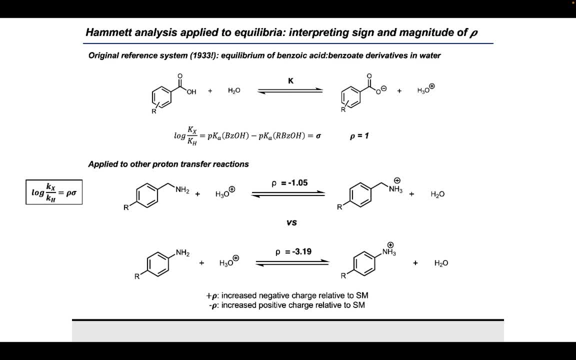 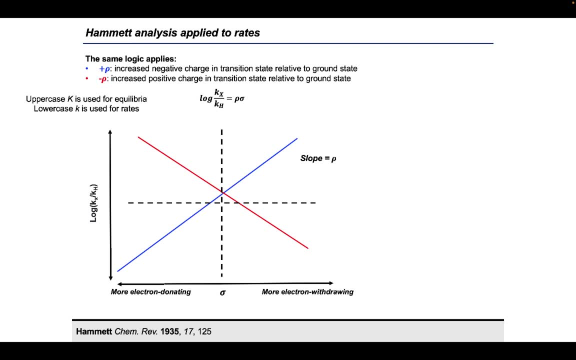 In these cases, we've looked at comparing two sets of equilibrium constants. However, I'd argue that the true utility of LFER analysis is applied to studying reaction rates, which allows us to leverage a reference reaction to give us a snapshot of the ever-elusive transition state. 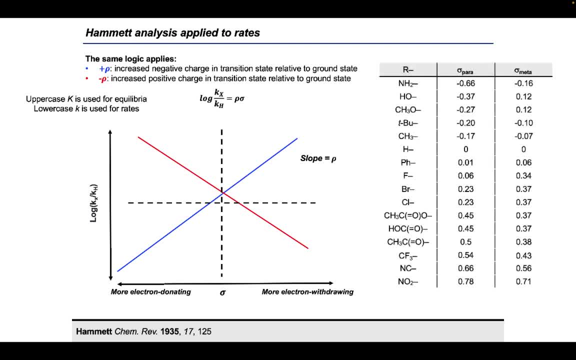 This analysis follows the same rules, of course, where if we observe a correlation with a positive rho value, this is indicative of increased negative charge in the transition state relative to the ground state, whereas if we see a negative rho value, this is indicative of increased 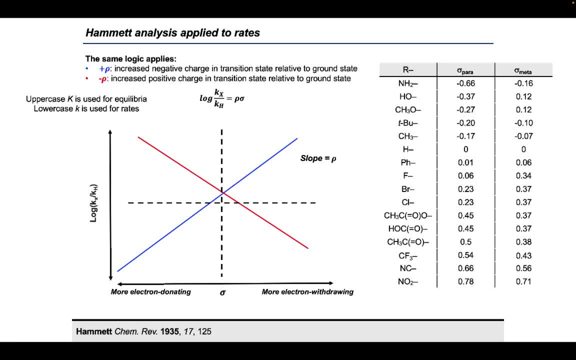 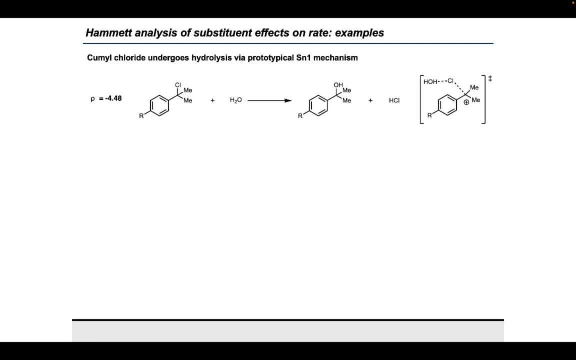 positive charge in the TS relative to the GS. Let's dive into some examples. Consider the substitution of the quaternary carbon as shown here. Let's consider a large negative rho, indicating that there is a great deal of positive charge developing in the transition state at the carbon attached to the ring. This is consistent. 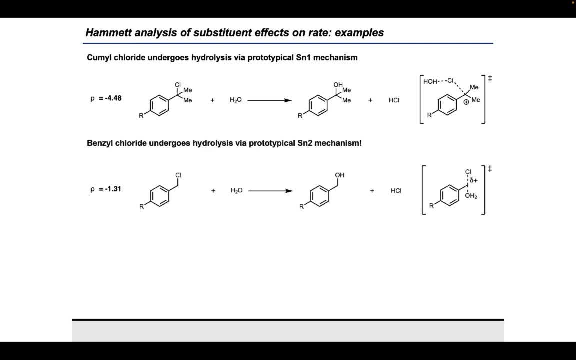 with an SN1 mechanism. Now, in contrast, in the substitution of the primary carbon, as shown below, we see a small negative rho. The negative rho still implies that there's buildup of positive charge at this benzoic carbon, but the smaller magnitude indicates that the amount of positive charge 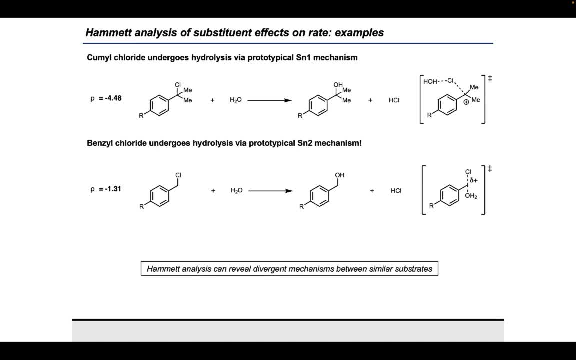 is relatively small, Pointing to an SN2-like mechanism in which bond breaking is more advanced than bond forming, thus making the carbon a little bit positive in the transition state. Now, while the standard Hamet sigma values are really useful, not all reactions correlate. 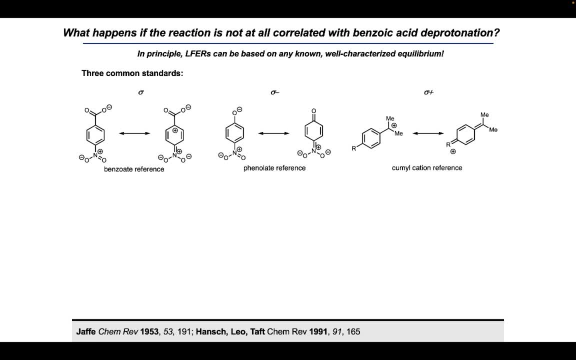 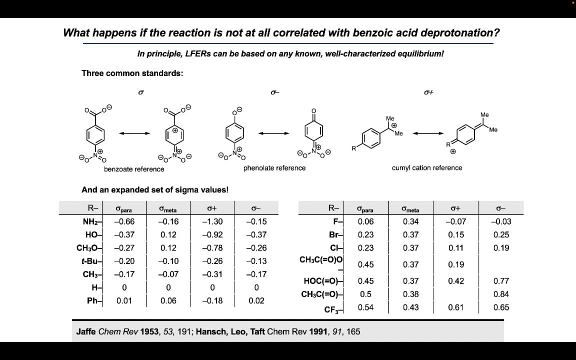 at all with the deprotonation of benzoic acid. Because of this, new Hamet parameters have been created, such as sigma-minus, which tracks the equilibrium of phenol deprotonation, and sigma-plus, which tracks the equilibrium of 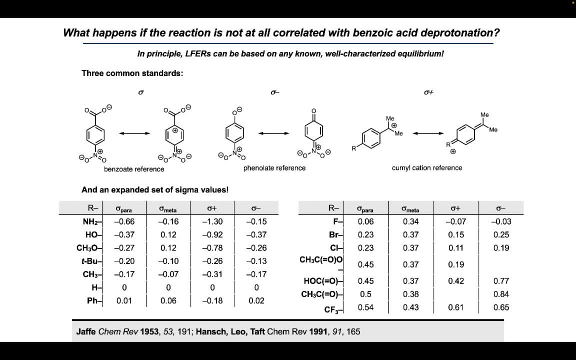 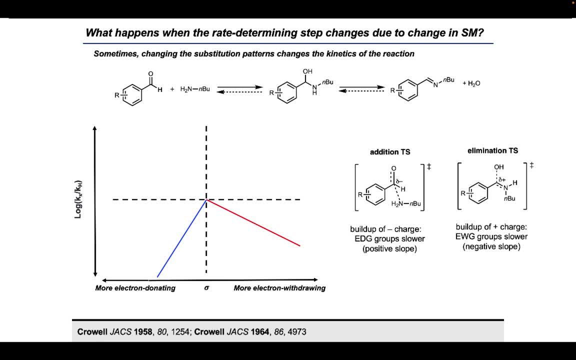 cumulocation formation from cumulocation. Now, as you might expect, sometimes the correlation is not linear throughout the entire range of substituent changes. This can happen when there are multiple steps in a reaction where changing a substituent changes which step has the highest energy. 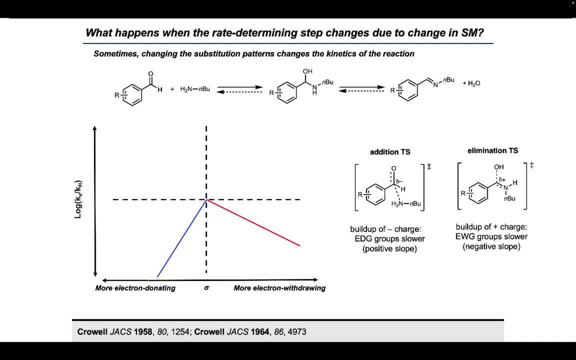 The example shown here is the formation of imines. In this case, we observe a plot with two regimes where each is linear, but with different slopes. A situation like this is down, where we have an inverted V-shape. Such a shape is signature for a change in the rate. 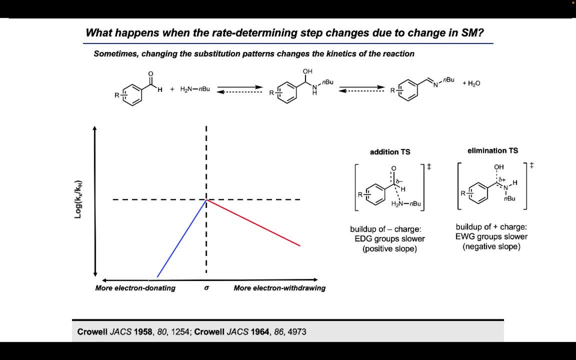 determining step. In the case of imine formation, there are essentially two steps: Formation of a hemi-amanal by attack of an amine on an aldehyde, and then breakdown of the hemi-amanal to generate the imine. 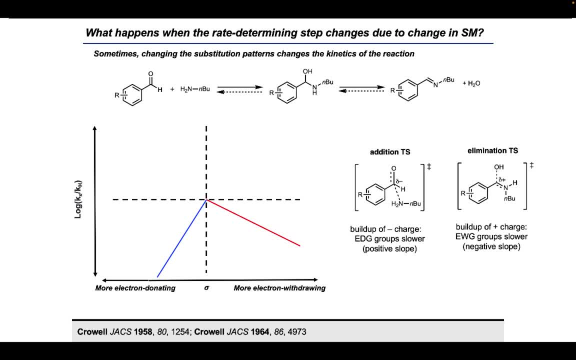 With electron donating groups, so those on the negative sigma value side, the aldehyde is more stable and the first step becomes rate determining. In this regime, decreasing electron donating nature increases the rate of the reaction. hence we see a positive slope. 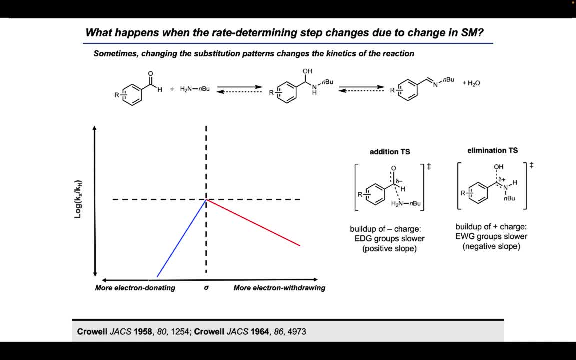 At a certain point though, in this case, where x equals h, we have made the first step so fast that the second step is rate determining. This second step now is made slower by electron drawing groups, and hence we see a negative slope in that regime. 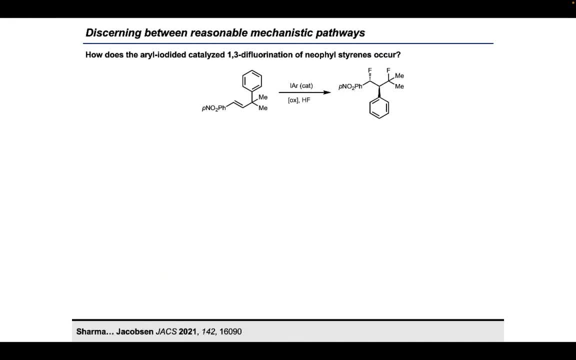 Moving on to even more complex settings, let's examine how we can use Hammett analysis to discern between multiple reasons. I will start by understanding the reaction of two Changstrahlers. A reaction in these省n지나-3-bluemilidea avec a shownwarts are called the. 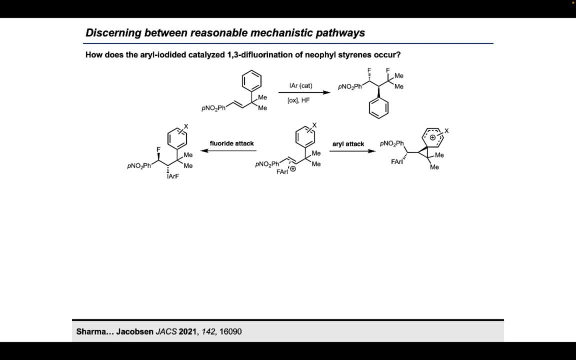 from a metal detection and a from a lugar detection. Either one will be THE reaction or both will be the reaction. The response can be a further reaction or a either-must-be reaction. Whether one is the reaction or the third one. The result is � p1,0 ,0,0,0 ,0,0 ,0 ,0 ,0,0 ,0,0,0 ,0,0 ,0 ,0,0 ,0,0 ,0,0 ,0,0 ,0,0 ,0,0 ,0,0 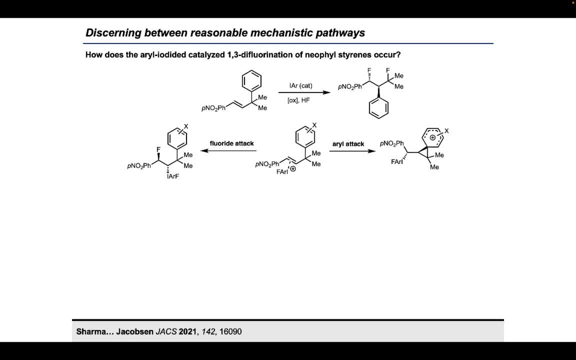 At what stage did this aryl group migrate? Did it happen after the alkene was fluoroiodinated, as precedent would suggest, Or did it happen first, before any fluorination in an aryl attack step? The key difference between these pathways is that in the latter case, 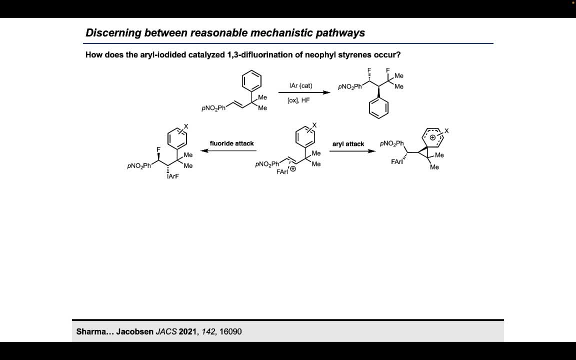 the aryl group builds up positive charge in what is likely the substrate committing step, Whereas in the former case the aryl group is not involved. So I measured the relative rates of substrates with differently substituted migrating aranes and what I found is that there is a huge correlation between the electronic nature. 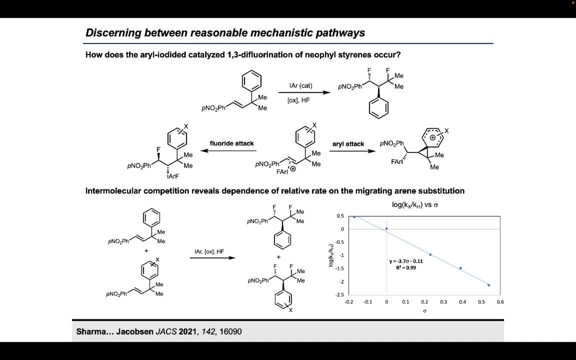 and the relative rates of the reaction, giving a rho value of negative three. This is consistent with an aryl attack first hypothesis and rules out the more commonly suggested fluoroiodination first pathway, allowing us to construct a more detailed mechanistic picture on this complicated reaction. 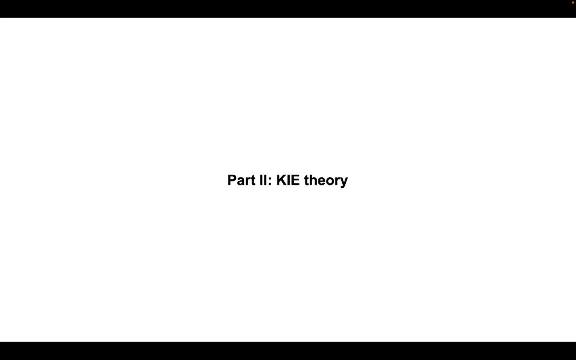 All right, let's move on to KIEs, which on the surface seem relatively different, but at the end of the day, it's all the same thing. A perturbation to the substrate allows us to measure a difference in equilibria or rate. 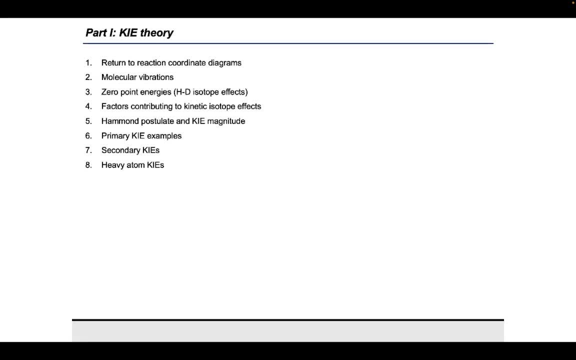 that tells us something about the mechanism. For this first half of the KIE lecture, I'll return to reaction coordinate diagrams and discuss the origins of isotope effects, namely how molecular vibrations cause changes in zero-point energies. Then we'll discuss how these phenomenon and other factors such as 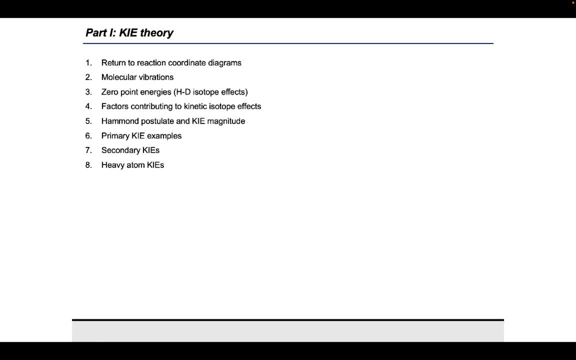 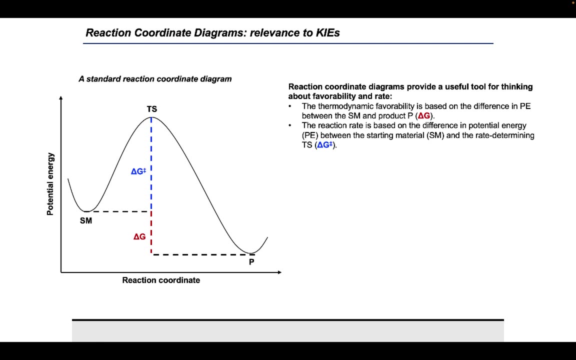 transition state position contribute to HD kinetic isotope effects. I'll run through some examples and then return to talk about carbon KIEs before we move to part two. Returning to the reaction coordinate diagram, we recall two different important measurements of potential energy changes: Delta-g, double dagger, which is the difference in energy. 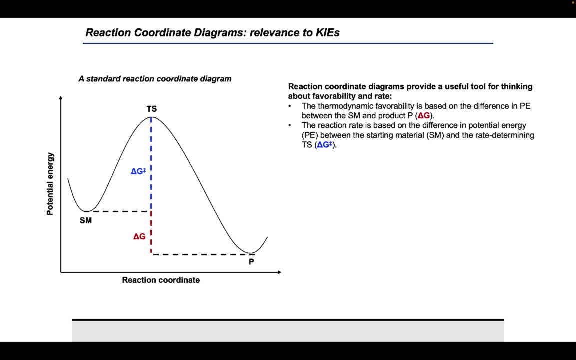 between the resting state and transition state and delta-g, which is the difference in energy between the starting material and product. There are two kinds of isotope effects that arise: equilibrium isotope effects which result from a change in delta-g between isotopically. 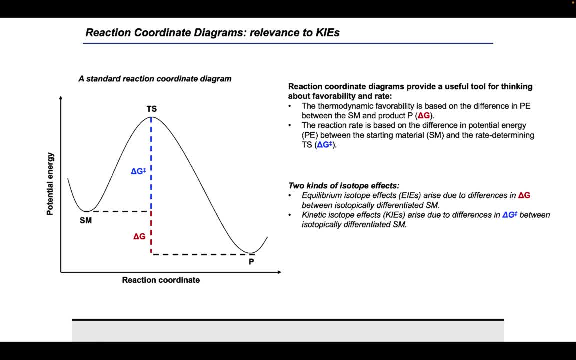 labelled substrates and products and kinetic isotope effects which arise from differences in delta-g double dagger between isotopically labelled substrates. Now, unlike in Hammet experiments, we can more safely assume that isotopic substitution does not change the mechanism of the reaction under study. 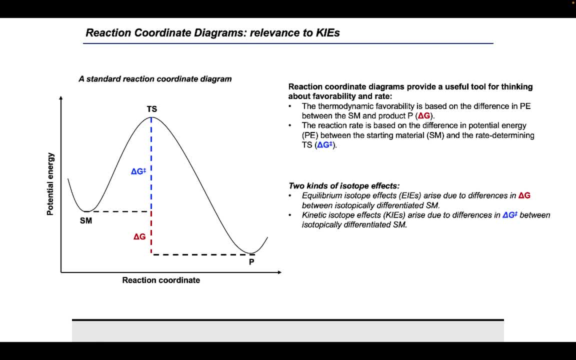 This is because isotopes only differ in the number of neutrons, and so we know that isotopic substitution doesn't change charge, and therefore we assume that there are no changes to electronic structure and thus no changes to the potential energy surface of the reaction. So how does 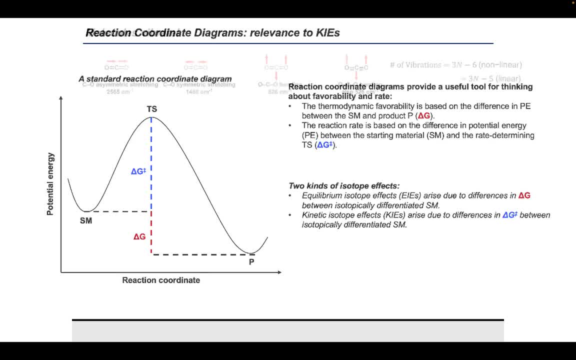 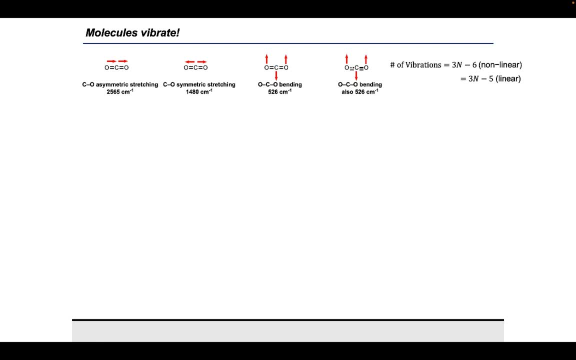 isotopic substitution affect reaction rates. It turns out, bonds vibrate, as we all know, and they do so at discrete frequencies. By vibration I mean molecular motions where the center of mass does not move. Now, what are the implications of this, If you look at this energy? 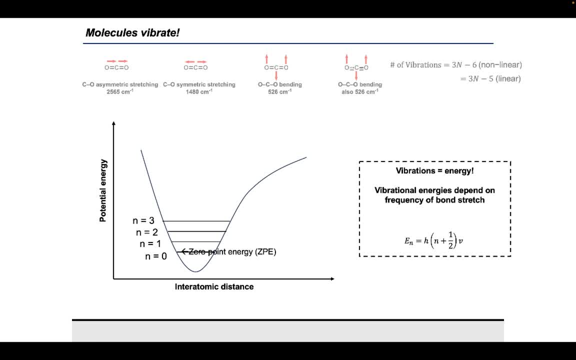 diagram. molecules do not reside at the bottom of wells on potential energy surfaces. Instead, they reside at slightly higher energy levels, depending on the energy present in the molecular vibrations. If n is the number of atoms in the molecule, linear molecules have 3n-5 vibrations. 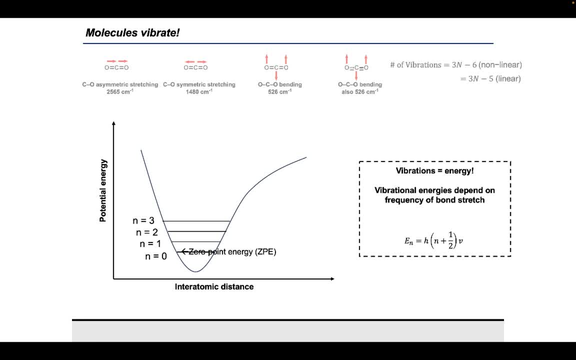 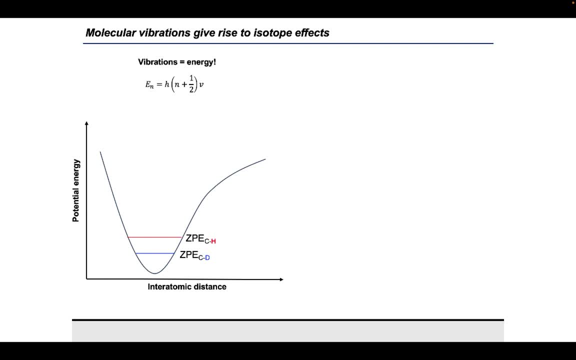 and all other molecules have 3n-6.. The vibrational frequencies can be represented in a Morse potential. Each vibration has associated energy levels, whose energies are provided by the formula shown above. The lowest energy associated with a vibration is obtained when we set n equals zero in the 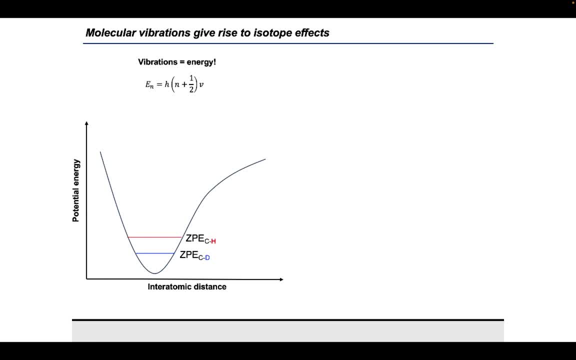 equation. This is called the zero-point energy ZPE, the key term and this is the state at which the vast majority of bonds are present. Consider a prototypical CH bond. The vibrational frequency for a CH stretching is 2800 wavenumbers. The ZPE associated with this stretching vibration 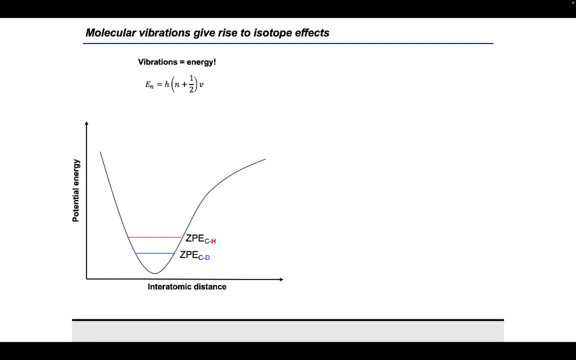 can be calculated from that value to be around 4kcal per second. The ZPE associated with this stretching vibration can be calculated from that value to be around 4kcal per second, and this is defined by ZPE per mole. 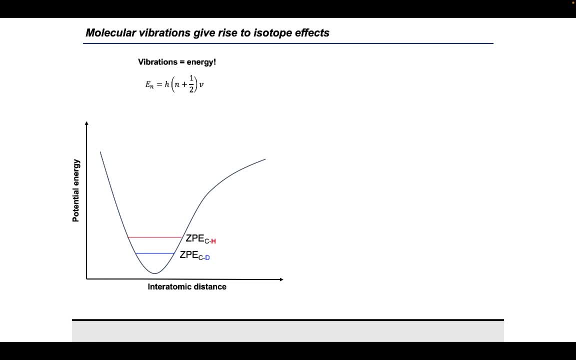 the second highest energy state for this vibration is 8kcal per mole. This essentially means that far less than 1% of molecules exist anywhere besides the ZPE. The frequency of bond vibration can also be expressed as a function of Hooke's law, ie. 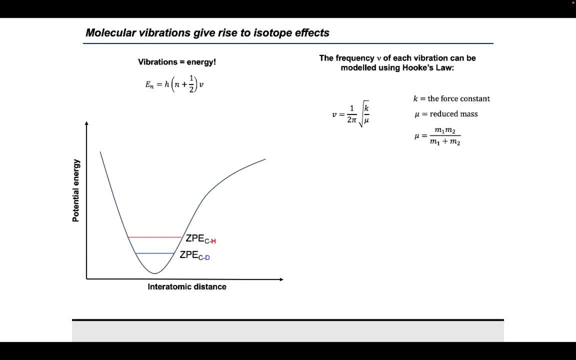 a spring of a given strength, n, with masses at the end, a force constant. K is a measure of how strong the bond is. Stronger bonds have higher values for K. The reduced mass values are calculated as shown. It depends on the masses of both. 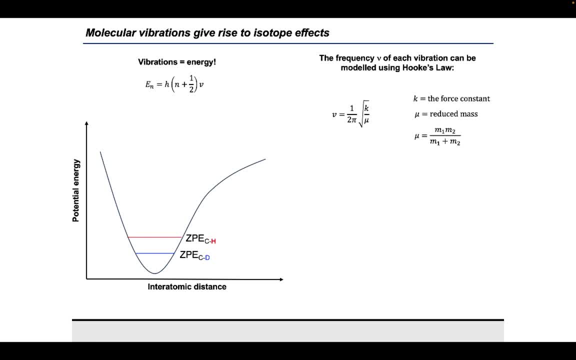 bonds at random. Second-highest energy state for a CH Tech ereależy from the ZPE, This credit of both atoms involved in the bond. So upon making an isotopic substitution in a bond, the force constant remains the same but the reduced mass changes As shown in this table. 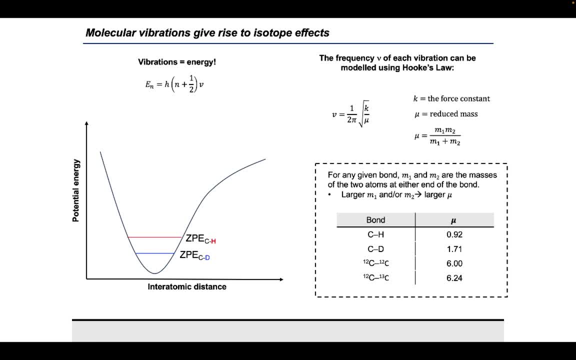 we see that the reduced mass for a C-D bond is nearly twice that of a C-H bond. Now the effects of isotopic substitution on reduced mass do get smaller with heavier atoms, as you can see here. From these results we can see that isotopic substitution leads to a 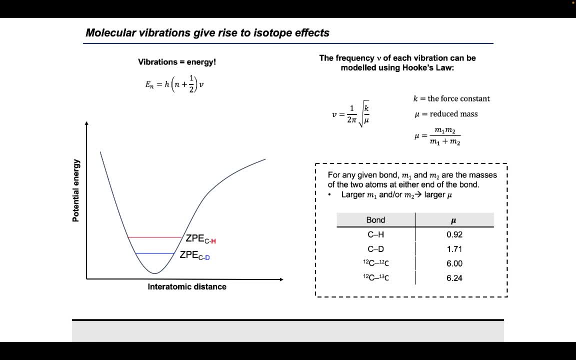 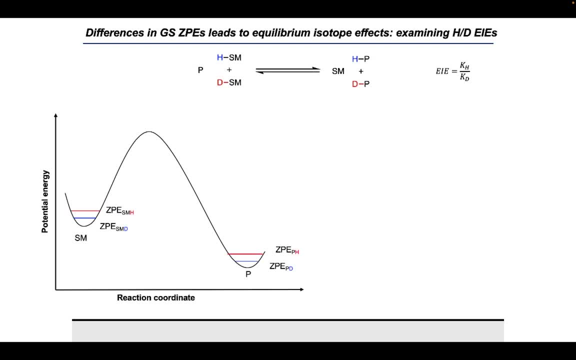 change in the Z-P-E associated with a bond. Particularly substituting an atom with a heavier isotope will decrease the Z-P-E. Now let's consider an equilibrium process. The equilibrium isotope effect is simply the ratio of equilibrium constants for the two. 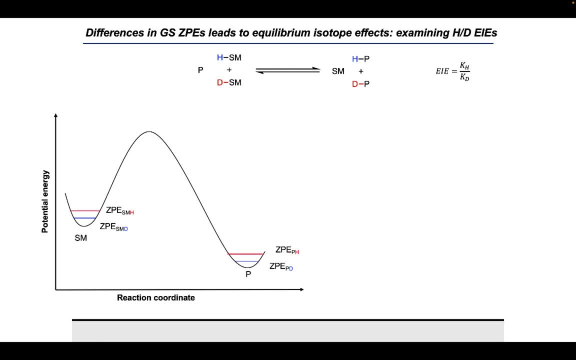 isotopologues. Let's consider two scenarios. In the first scenario, a compound with a stronger bond is being replaced by a product with a weaker bond. As the difference in Z-P-E between compounds with H versus D substitution is proportional to the force constant, the delta Z-P-E is greater in the starting materials than in. 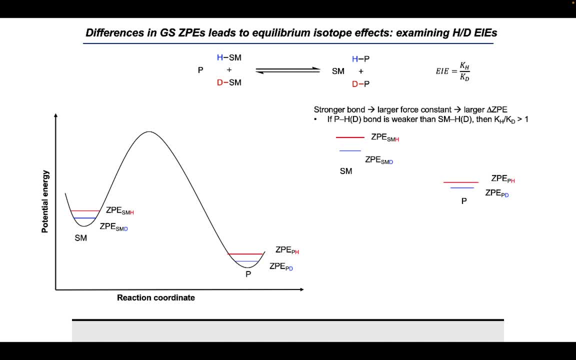 the product. This results in a greater free energy difference, delta G for the H-containing molecule and going from starting material to product, as shown here. Consequently, K-H is larger than K-D and we observe a normal E-I-E. 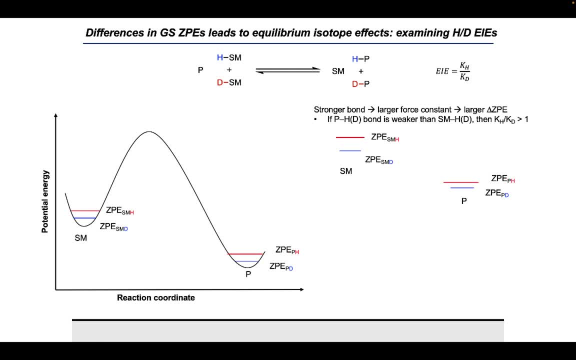 The analogous situation where a weaker bond is replaced by a stronger bond in the product is shown in this lower scenario. In this case, the E-I-E is inverse In general. remember that the heavier isotope will always prefer to be in the stronger bond. 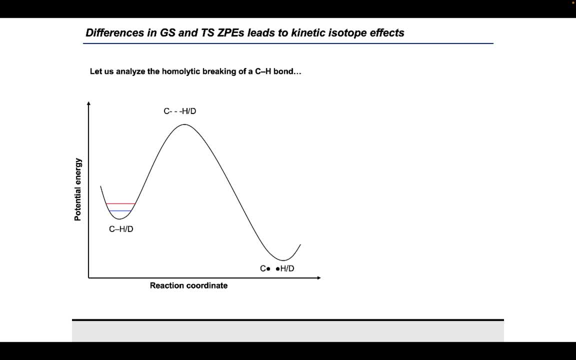 Now let's think about how isotopic substitution could affect reactivity. Consider the homolytic dissociation of a C-H bond, aka the process of stretching this bond so as to give independent C and H atoms, each with one electron from the bond. 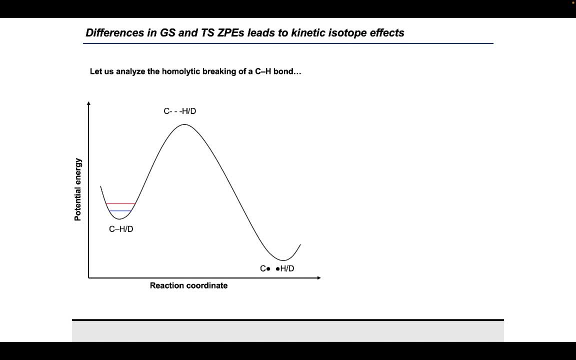 The potential is shown in the graph. The C-H bond resides in the red energy level and the C-D bond resides in the lower blue energy level. Because there is no change in the potential energy surface due to isotopic substitution, both bonds have the same potential curve. 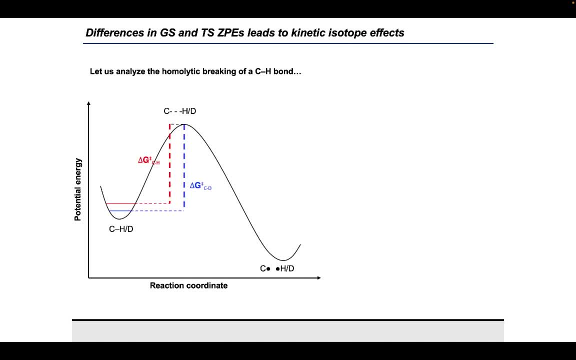 The energy required to break the C-H and C-D bonds is shown in red and blue respectively. The C-D bonds start to break the C-H bonds and C-D bonds start to break. the C-D bonds start from a lower energy and therefore it takes more energy to break that C-D bond. 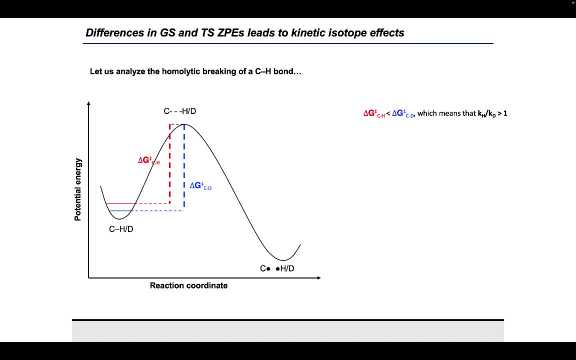 The difference in activation energies is exactly equal to the difference in ZPEs. We can calculate rate constants from these energies using the Eyring equation. We then arrive at a Ke of approximately 6.8 at 298 Kelvin. This is the Ke expected for. 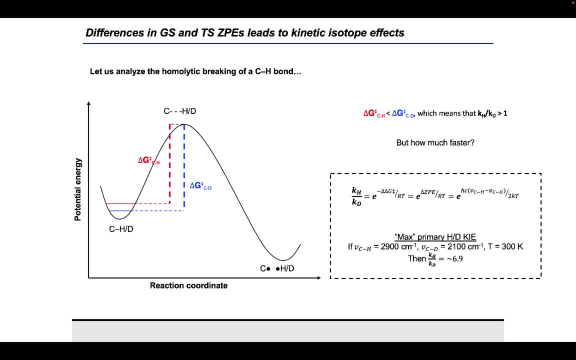 bond homolysis of a C-H bond. As we'll see later on, this is the maximum possible HD Ke, Although there can be some funny business that we'll talk about too, When a Ke is measured at an atom to which a bond is being broken or formed in the transition. 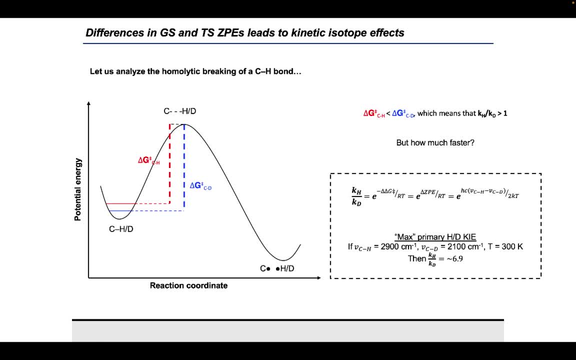 state, it is called a primary Ke. like shown here, Primary Ke's are generally greater than 1.3.. When a Ke is measured at an atom whose bond is not broken in the transition state, it is called a secondary Ke. Secondary Ke's are usually between 0.75 and 1.3.. We'll 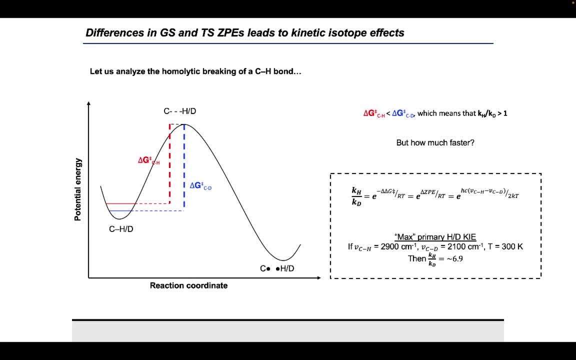 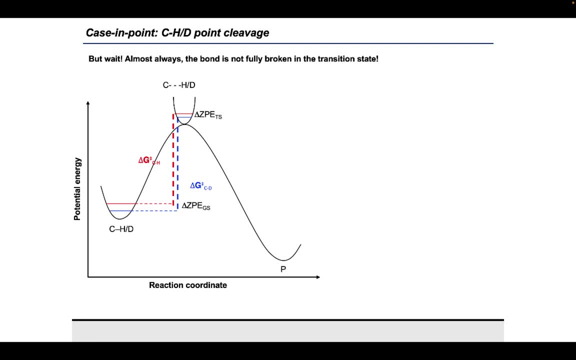 talk about these more later, But first let's add an important complication. The vast majority of reactions are not simple homolytic dissociations. Instead, bond breaking and forming is only partial in the transition state. Weakening of bonds results in smaller yet still existent force constants, Because 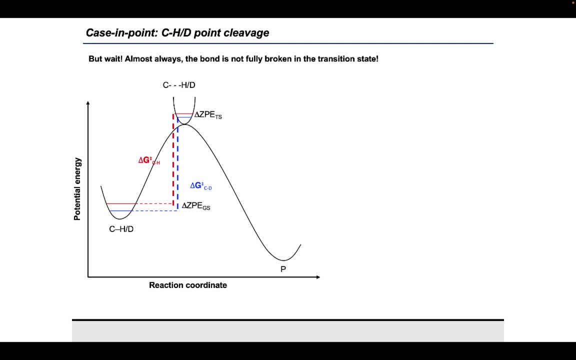 the force constant changes. in going from starting material to transition state, the delta ZPE also changes. comparing the starting material to transition state structure Specifically, the delta ZPE is generally smaller in the transition state than in the starting material. The difference in rates is thus related to this difference in delta ZPEs. 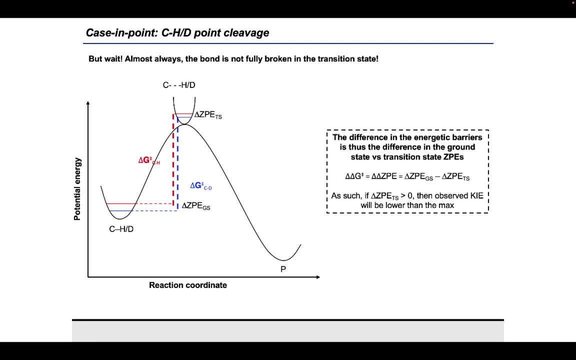 Reactions that feature minimal change in ZPE going to the transition state versus the ground state will display Ke's in the smaller 1 to 6 range. Reactions that decrease dramatically in ZPE in the transition state will display much larger Ke's with a theoretical maximum. 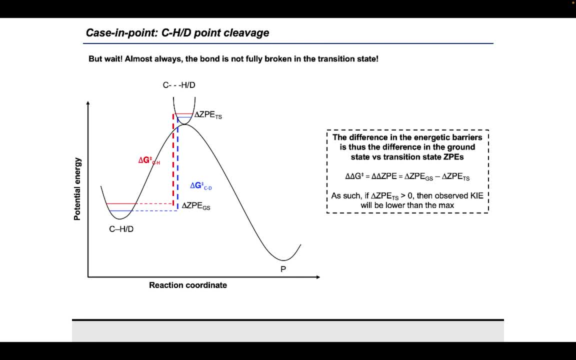 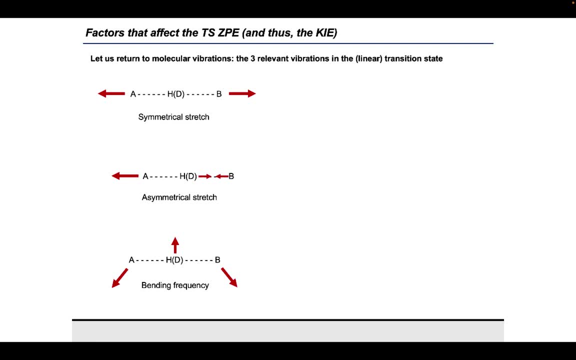 being 60.. Now, what are the factors that control the transition state ZPE? Obviously, it's the vibrations. To think about this, let's consider a simple reaction involving hydrogen atom transfer between A and B. The species in the transition state has 3 and minus 6, aka 3, vibrations. 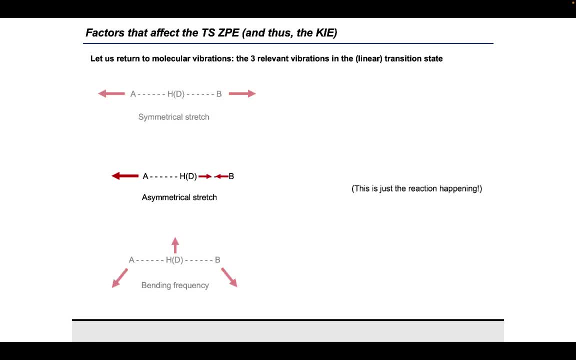 These three are shown here. The asymmetric stretch is the reaction coordinate and doesn't contribute to the ZPE difference. Bending frequencies are, as a general rule, small than stretching frequencies and therefore contribute little to the ZPE difference. This leaves the symmetric stretch. This stretch is the main contributor to the delta ZPE of. 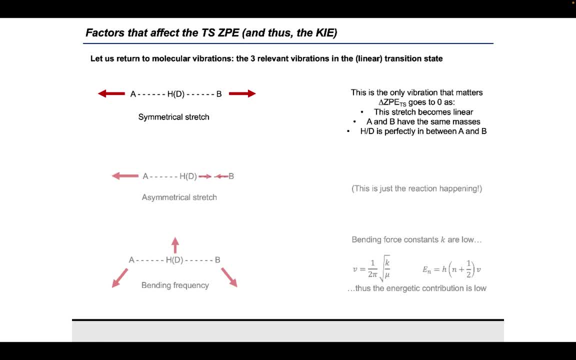 the transition state. The more vibration there is in this stretch, the larger the delta ZPE will be, and so we can expect the things that decrease the amount of vibration or movements will decrease the ZPE and thus maximize the observed Ke. There are three main things here that will. 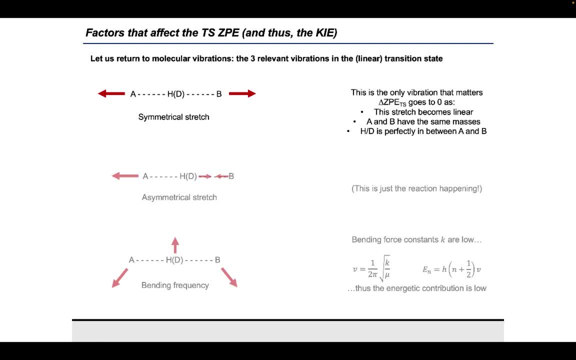 affect the amount of vibrations in this stretch. So if this stretch is linear, that minimizes the amount of vibrations. If A on one hand and B on the other hand of the H atom are the same masses, that will also decrease the amount of vibration. And then, finally, if 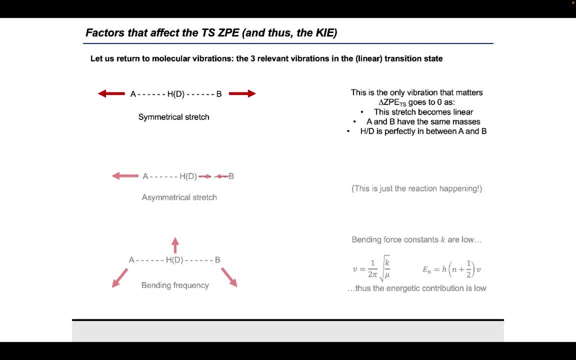 H or D is right perfectly in between A and B, then there will be a very small amount of ZPE difference. For this reason, it should not be surprising that the position of the transition state between the starting material and the transition state will be the same. This is because the 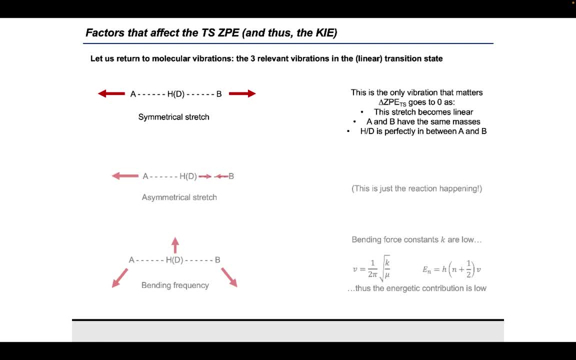 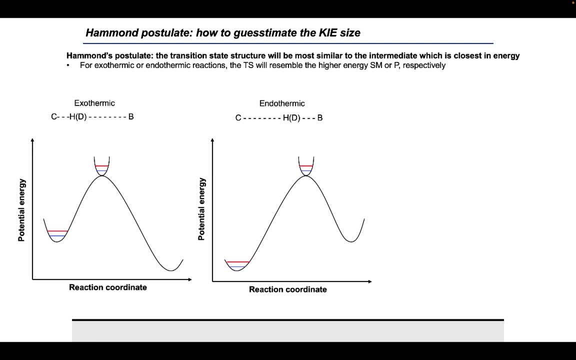 starting material and product along the reaction coordinate will have a direct effect on the magnitude of the Ke. Recall that the Hamann-Pauschelit dictates that when a reaction is exothermic or endothermic, the transition state is earlier or late respectively. 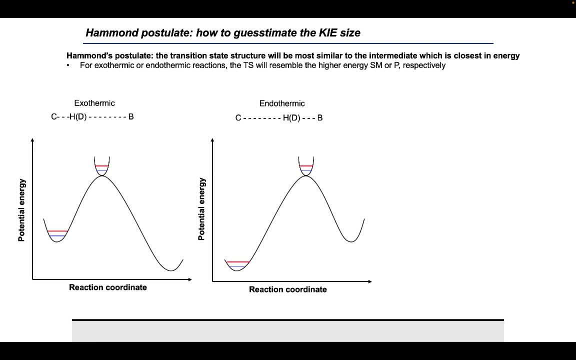 In these cases, the transition state is not symmetric, So the symmetric stretch is expected to involve a lot of motion of the central atom, And so we would expect a relatively small Ke. However, for a thermoneutral reaction, this is a small Ke. This means that the transition state is not going to change the direction, but the Ke is going to be the same. So the B in general would be the same. I aside this, the C in other case speaks for the same point. The B is going to be the same. However, for a thermoneutral reaction the land is going to be a little bit more independent. 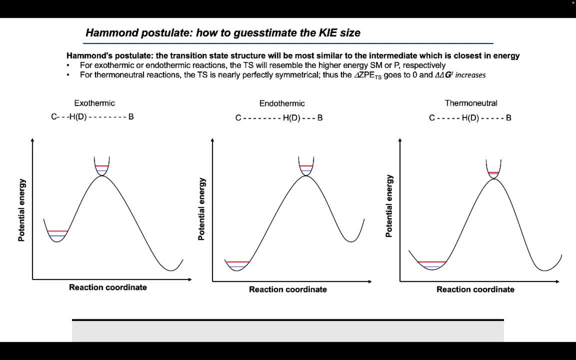 we would expect a transition state to be much more symmetric, with limited motion of the H-atom and therefore a much larger KIE, because there is really no delta-ZPE in this transition state. Now that we have discussed the theoretical aspects that govern the magnitude of KIEs, 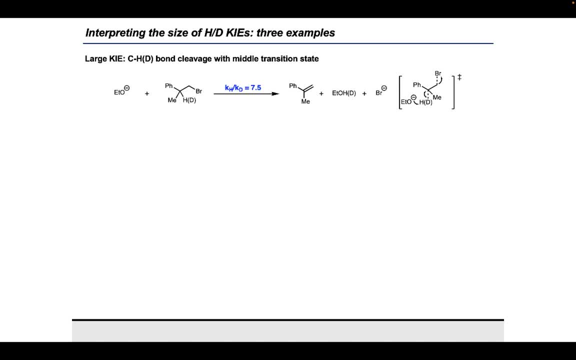 let's look at some examples to understand how to interpret the magnitude. The first example is the typical E2 elimination reaction, in which depronation occurs at the same time as bromide displacement. We see a primary KIE of 7.5, which is consistent with C-H bond breakage in the transition state. 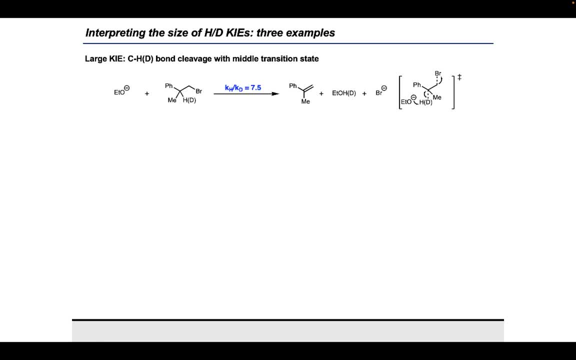 The magnitude suggests that the reaction has a transition state that is neither early nor late. The second example is also an E2 reaction, but we have replaced the bromide with trimethylamine. This is a much better leaving group and as such, we would expect an earlier transition. 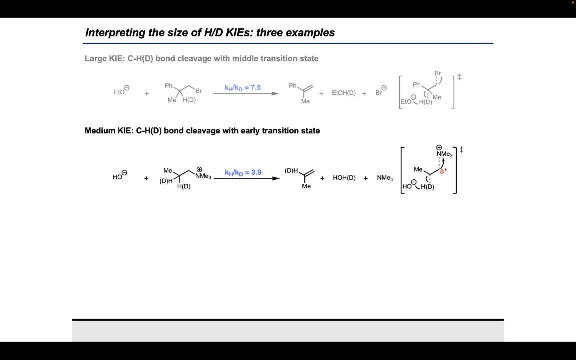 state. Consistent with this, the observed KIE is 3.9,, which is a primary KIE. that indicates C-H cleavage in the transition state, but is much smaller than the 7.5 because this transition state is so much earlier. 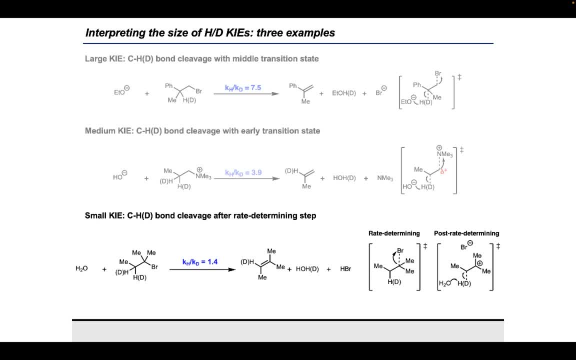 The final example is an E1 elimination reaction where we observe a KIE of 1.4.. This number is much too small to be a primary KIE and is indicative of C-H cleavage occurring after rate-limiting CBR heterolysis. 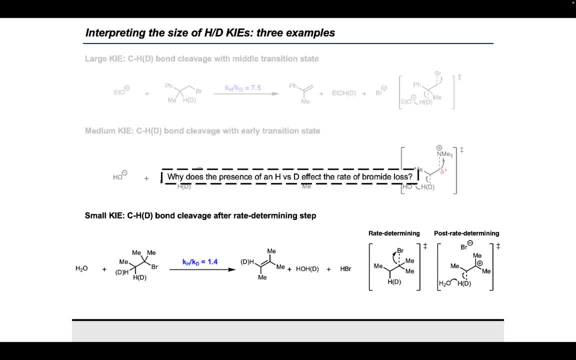 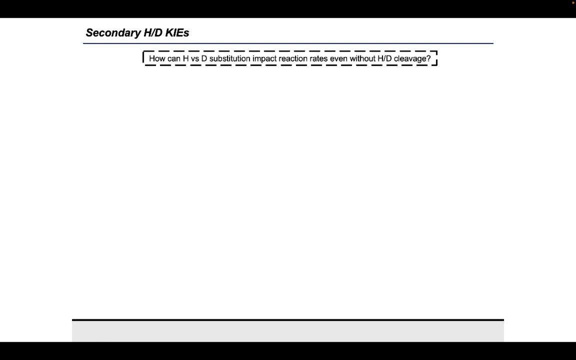 Interestingly, though, this number is not 1.. How could that be? So far, we have discussed the interpretation of primary KIEs, that is, KIEs measured at atoms that are undergoing bond breaking or bond forming. However, it is also possible for isotopes to have an effect on rate when they are not. 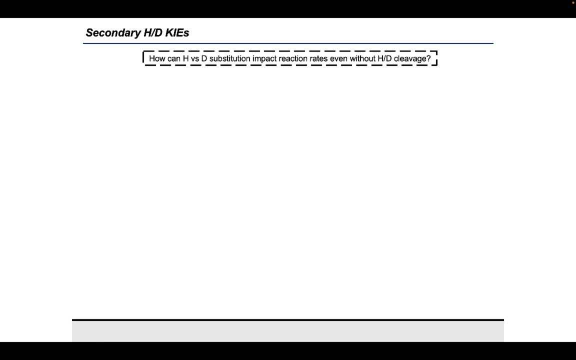 undergoing direct bonding changes. The KIE measured on such an atom is referred to as a secondary KIE. Secondary KIEs are generally measured on hydrogen atoms, and that's what we'll talk about today In this example: hyperchloride. 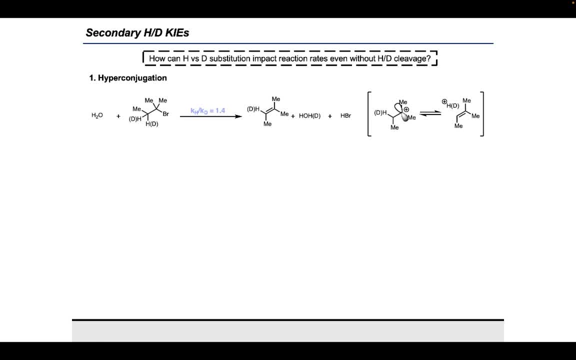 Hyperconjugation results in a normal KIE. that's small but still significant. Hyperconjugation weakens the vicinal C-H-C-D bonds and thus lowers their associated vibrational frequencies, which results in a slightly smaller delta-ZPE in the transition state and thus 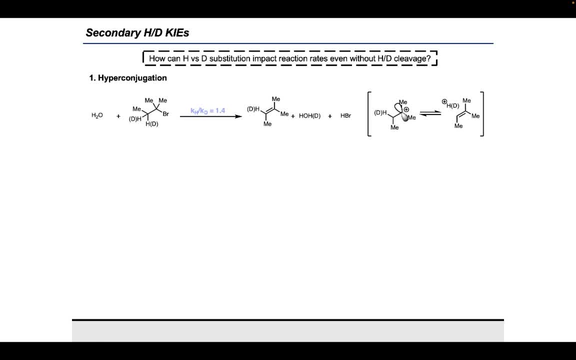 leads to a small KIE. Additionally, since the deuterium-labeled molecule has a stronger bond to carbon, it participates in this hyperconjugation to a lesser extent than the proteated molecule, giving a small, normal KIE again. The second reason we see secondary KIEs, which is maybe more common, is because of re-hybridization. 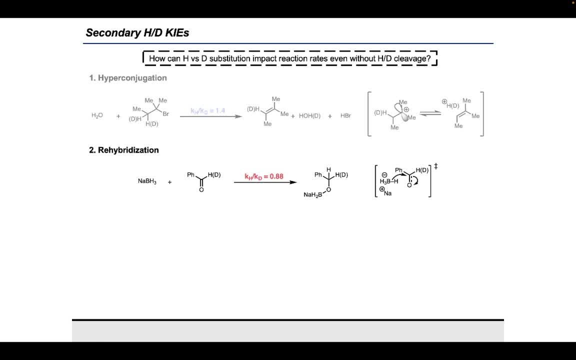 effects. Let's look at an example. Examining the reduction of benzaldehyde with sodium borohydride gives a KIE that's actually smaller than 1.. In this case, the deuteroaldehyde reduces faster than the proteoaldehyde. 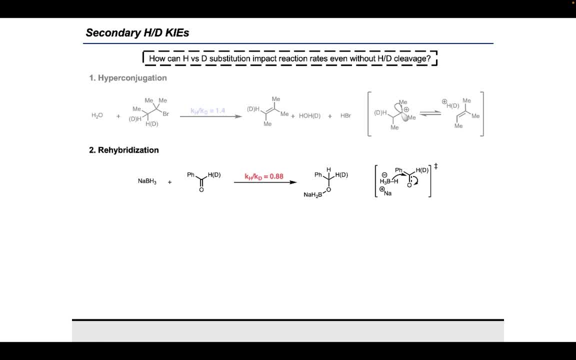 Again, the proton in question does not experience bonding changes in the transition state. However, there is a change in the hybridization of the carbon bearing the proton in going from the ground state to the transition state. This can be explained again by going back to our knowledge of molecular vibrations. 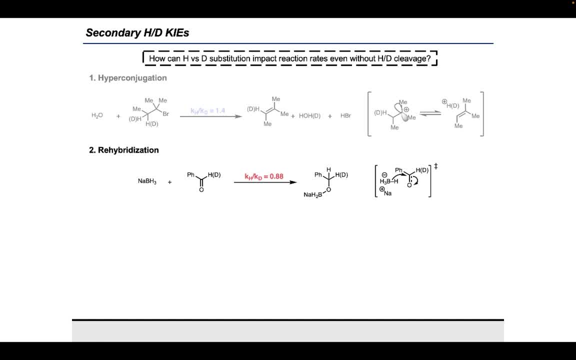 Stretching frequencies in this case do not change significantly when the bond in question is not broken or formed in the transition state. so there must be some other contributor here. It turns out that bending frequencies associated with C-H bonds can undergo a significant change. 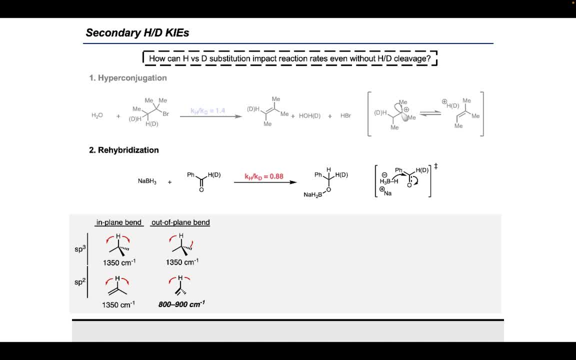 when the hybridization of the carbon changes. I hope you enjoyed this video. There are two primary bending frequencies to consider: an in-plane bending mode and an out-of-plane bending mode, as illustrated in the box below. The in-plane bend does not change in going from sp3 to sp2.. 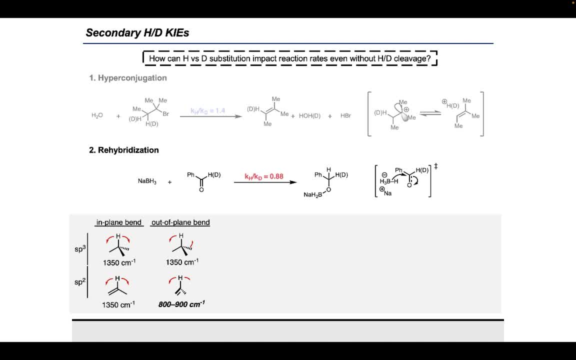 However, the out-of-plane bending mode is significantly reduced in going from sp3 to sp2 hybridization. This results in a difference in delta-ZPEs when the carbon attached to the desired proton undergoes re-hybridization in the transition state. 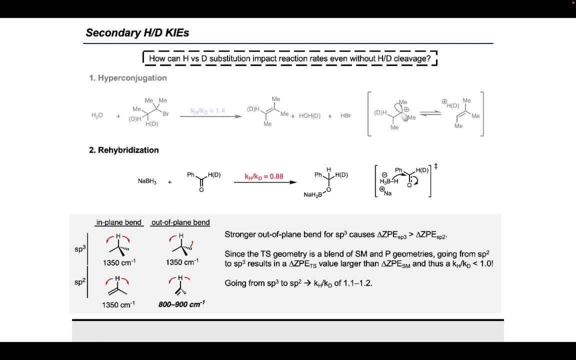 This change in delta-ZPEs is what causes the observed secondary KIE. Notice that the bending frequency is greater in the sp3 hybridized carbon than in the sp2 hybridized carbon. This means that a change in hybridization from sp3 to sp2, in going from the ground, 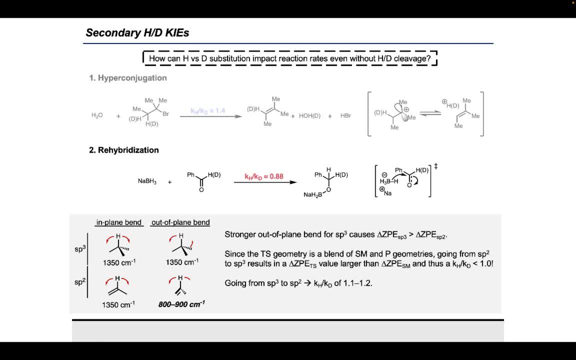 state to the transition state will result in an inverse secondary KIE. less than 1.. A change in hybridization from sp2 to sp3 in going from the ground state to the transition and going from the ground state to transition state will result in a normal secondary KIE. 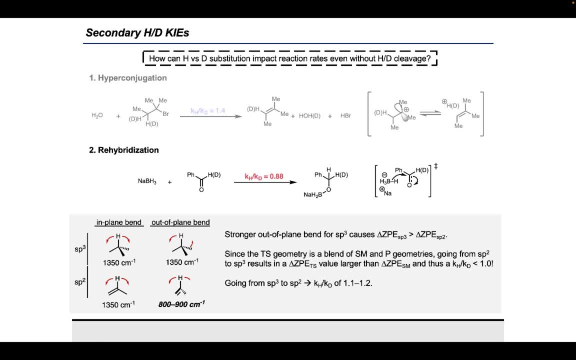 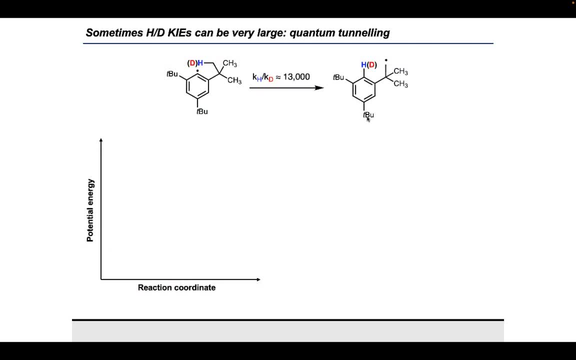 And so the range of these KIEs is about 0.75 to 1.3. Now, thinking about the opposite end of things, sometimes measured KIEs are surprisingly large. Recall that we said that the maximum theoretical HD KIE was 6.8.. 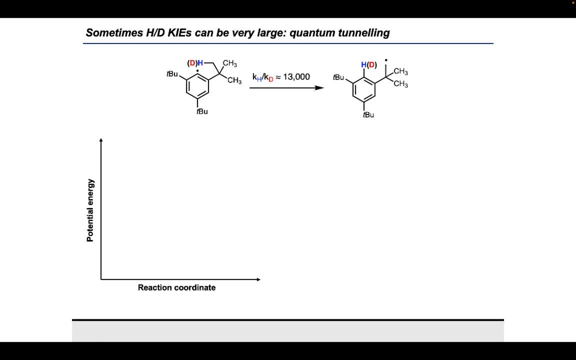 And the example shown on this slide was an HD KIE of 13,000.. How is this possible? This has to do with a quantum mechanical effect called tunneling. Think of a reaction coordinate as two intersecting parabolas, as shown below. 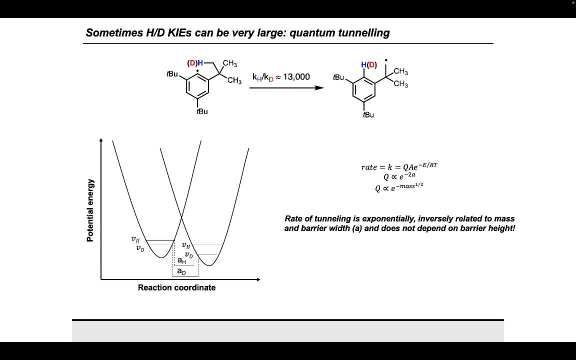 According to Marcus' theory, we can think of starting materials going up from one parabola until they reach the intersection between the two parabolas, at which point they can go down the second parabola to form a product. This way of thinking is not so different than the reaction coordinates that we've seen so far. 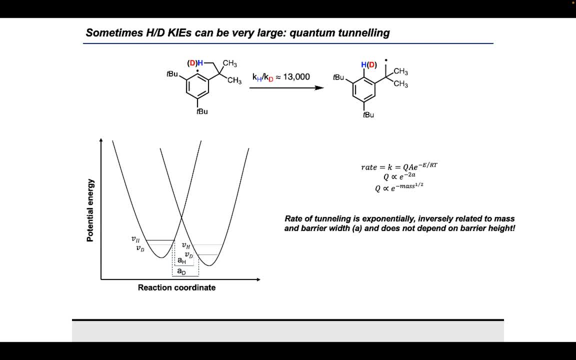 The intersection is the transition state. The bottom of the wells are just the ground states, So it's just a slightly different portrayal. However, the mathematics of quantum mechanics, which I am not going to get into, tells us that there is a finite but very small probability. 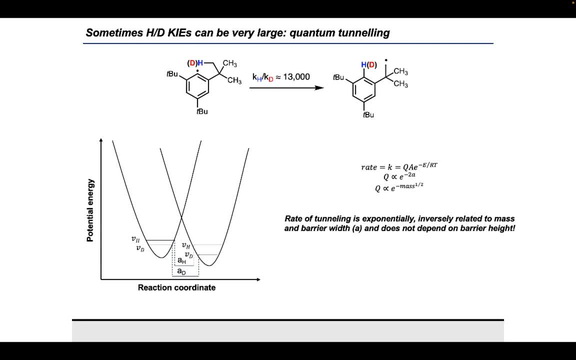 of finding a particle that should be in the first parabola but is in the second parabola. This effect, by which a particle can move from one energy well to the other without passing through the transition state, is a form of tunneling. 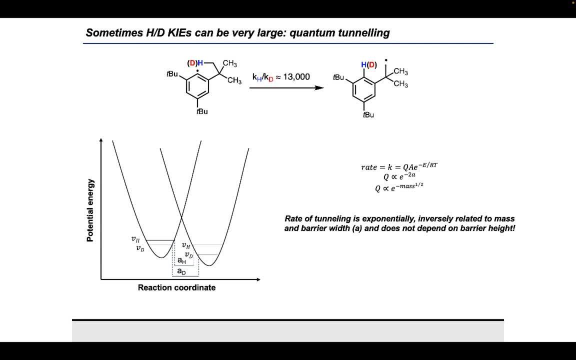 The tunneling rate depends on the barrier width and the mass of the particle. Smaller barriers result in more tunneling. Smaller masses result in more tunneling. Thus H can tunnel exponentially more than D can. This can underlie sometimes extremely large KIEs. 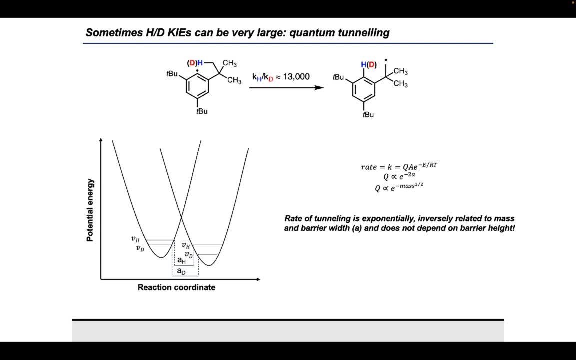 Any KIE greater than 10 is usually ascribed to tunneling. Any KIE greater than 10 is usually ascribed to tunneling. Any KIE greater than 10 is usually ascribed to tunneling. Note that these tunnelings don't depend on barrier heights. 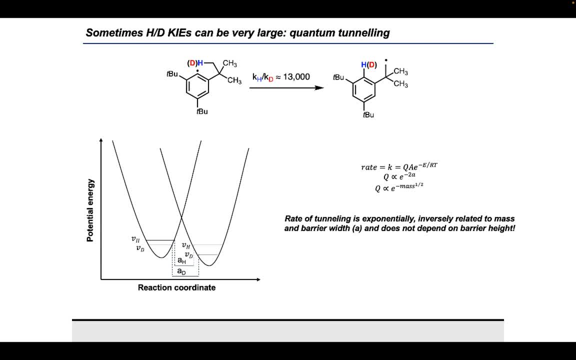 which means that the rates of tunnelings are independent of temperature. So if you suspect that there is tunneling in your KIE, to confirm this you can take the KIE value at many different temperatures. If the value doesn't change, it's likely due to tunneling. 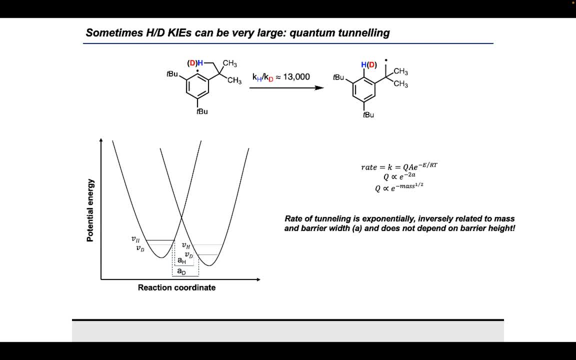 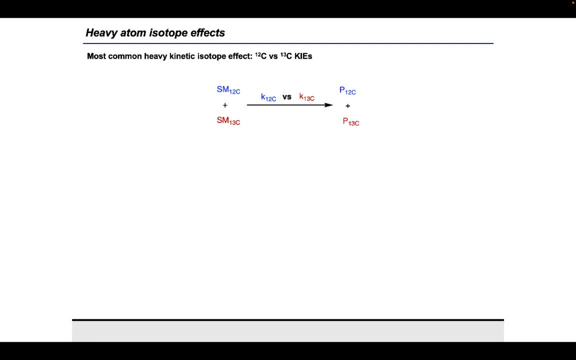 But also, if you are getting a value of 1000 or something anyways, then you have little to question. Up to this point, Up to this point, we've only really talked about HD KIEs. but there's a much broader range of KIEs. 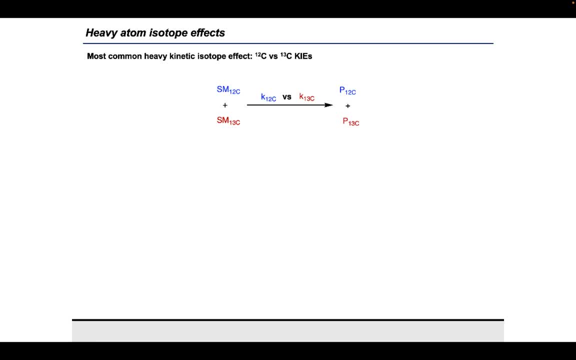 that are useful for mechanistic analysis. Before moving on, I want to introduce carbon KIEs Now. a typical primary KIE at carbon- comparing carbon-12 and carbon-13, is around 1.02 to 1.07,. 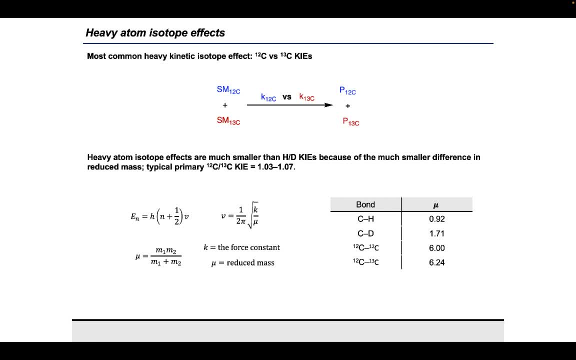 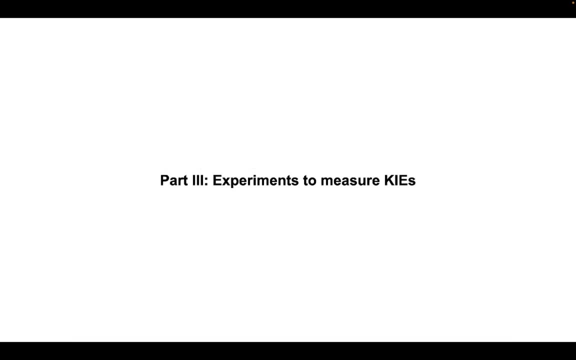 which we also maybe call a 2% to 7% KIE. Because these numbers are so small, they can be quite difficult to measure accurately and precisely. so we'll get into that at the very end of the next section. All right, so now it's time to put the theory we've learned into practice In this next 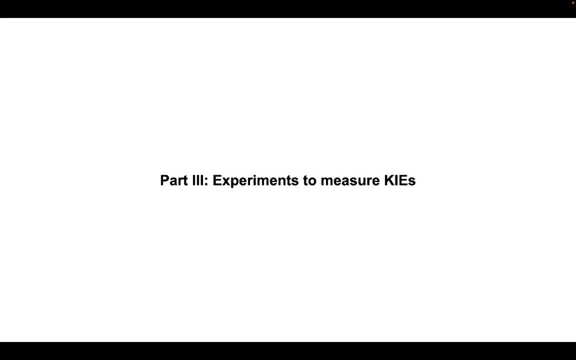 section we'll discuss different types of experiments to measure KIEs. But don't worry, this will be much more than nitty-gritty. We're going to learn how to think like a mechanistic chemist. All right, there are several methods by which people measure KIEs. The first is absolute rates. 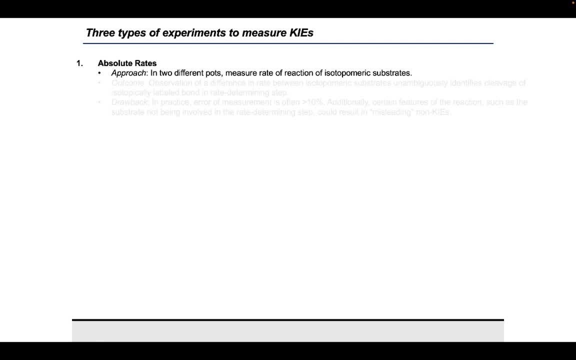 or just measuring the two rates of reaction of isotopomeric substrates in different pots. Secondly, there's intermolecular competition. This involves mixing two isotopomeric substrates in one reaction flask and observing the relative rates of the substrates. 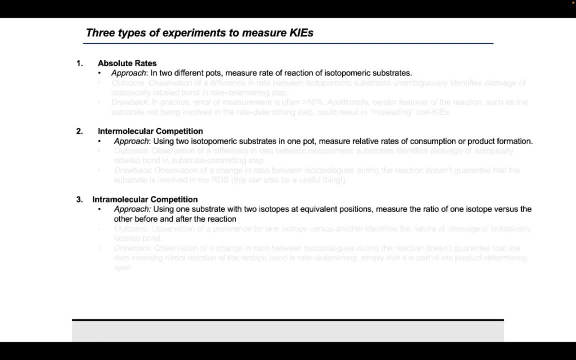 And then, finally, there's intramolecular competition. This involves using a single substrate with two isotopes that are at equivalent positions on the substrate, where one of them could react preferentially over the other, of course, if involved in the reaction. In all of these, 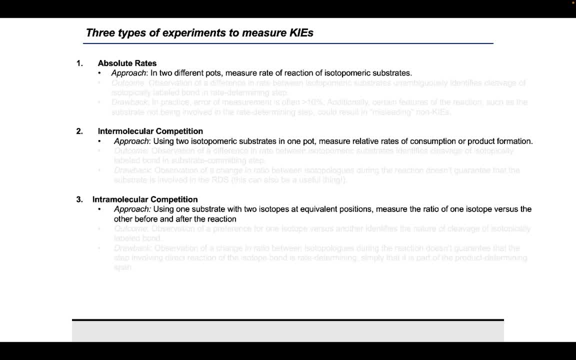 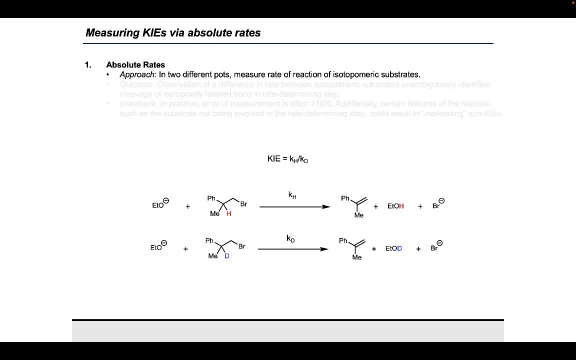 cases, it's most common to synthesize isotopically labeled starting materials for use in the studies. All right, number one: absolute rates. So in this case, as shown in the scheme below, this involves measuring the rate of two isotopically. 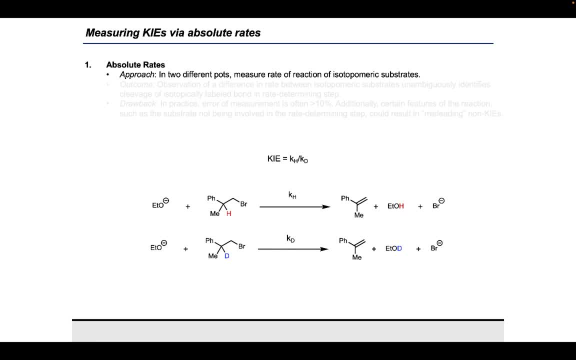 labeled substrates each in their own separate reaction flask. If we can observe a large KIE from these absolute rate experiments, this provides unambiguous evidence on a C-H bond breaking in the rate-limiting step. Now there are a few disadvantages or challenges to this method. 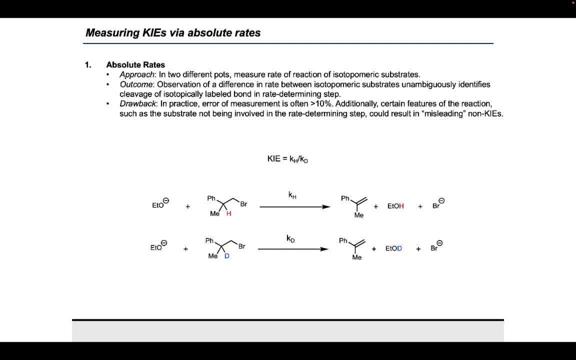 One of them is that measuring absolute rates requires doing kinetics, which can be difficult and prone to errors, often of at least 10%. Additionally, the rate-determining step of the reaction might not even involve the substrate, And so, regardless of C-H bond cleavage or not, 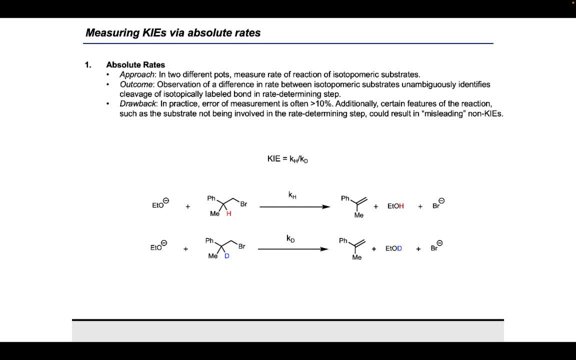 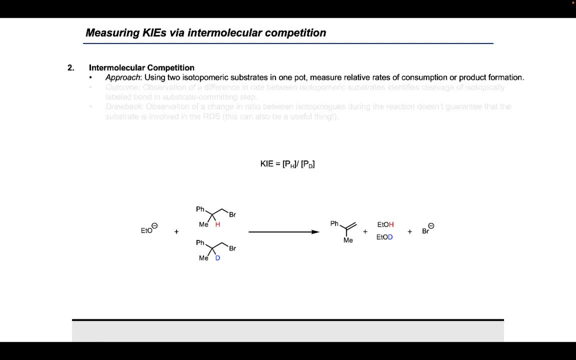 in those cases we wouldn't expect to see a KIE. We could instead measure a KIE by a competition experiment. In such an experiment, the differently labeled starting materials are combined and then subjected to the reaction conditions in the same pot. The reaction is taken to a. 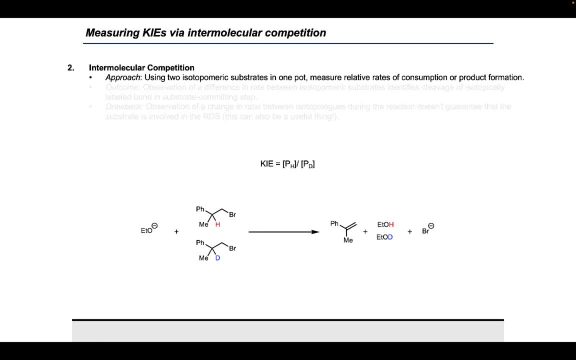 partial conversion and then the ratio of starting materials or products is measured. The ratio of starting materials or products can then be used to calculate the KIE. It's important to note that the observation of a large KIE from an intermolecular competition experiment does not necessarily mean that C-H cleavage takes place in the rate determining step. 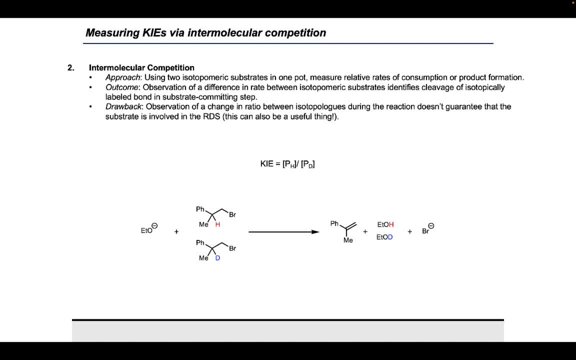 This is really just evidence of C-H cleavage occurring in the substrate committing step, But again, this isn't a great application, of which KIE is relevant here, as we'll strawberry take, Have the evidence later, But of course, the main reason why you might, in your case a 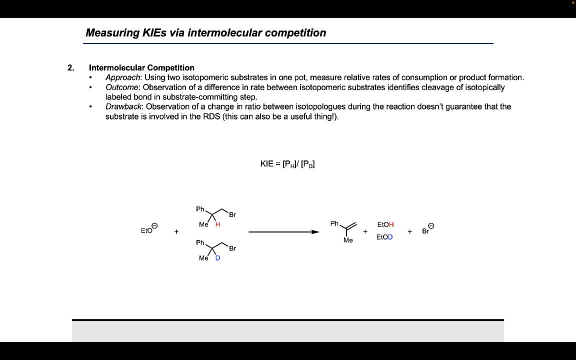 price. Finger substrate committing step is just the step where, once the substrate reacts in a certain way, it can no longer go back to starting material. thus it's committed. This method is much more advantageous because it doesn't require kinetics. it simply requires running the reaction of partial conversion. 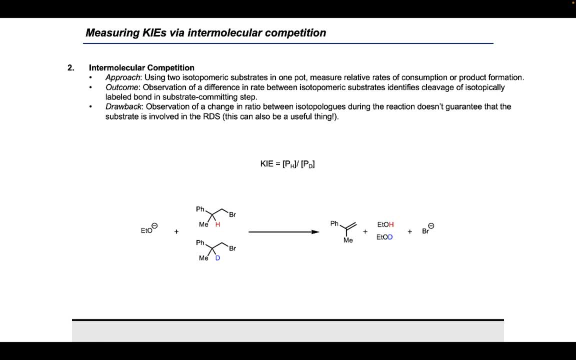 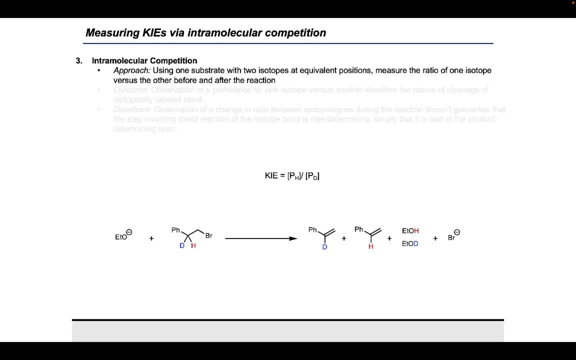 and then measuring ratios, As we'll discuss later. these ratios of products or starter materials is not exactly the KIE, but from the conversion and from this ratio we can calculate the KIE. A third experiment is intramolecular competition. In this experiment a molecule contains two. 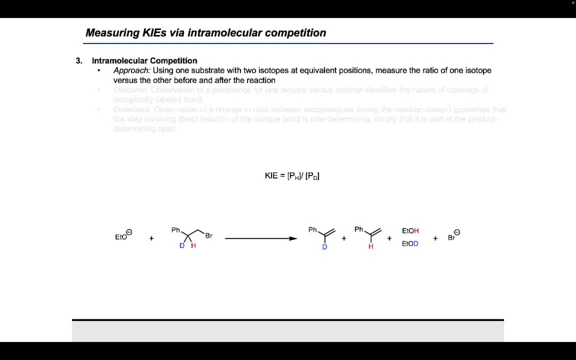 different isotopes in chemically equivalent positions. The ratio of products at any time point of the reaction directly provides the KIE. However, as with the intermolecular competition experiment, the observation of a large molecule is not exactly the KIE. but from the conversion. 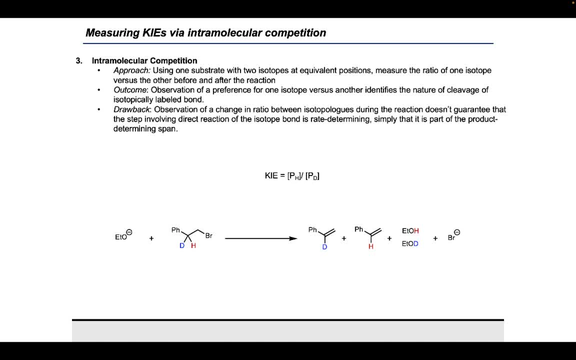 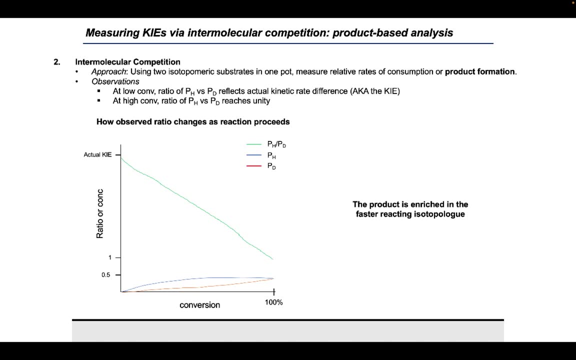 is shown differently. The increase in the KIE does not necessarily mean that C-H cleavage occurs in the rate determining step or, in this case, even in the substrate committing step, and so the results must be interpreted carefully. Now let's consider a reaction that, say: has a KIE of 5. The green line here plots the 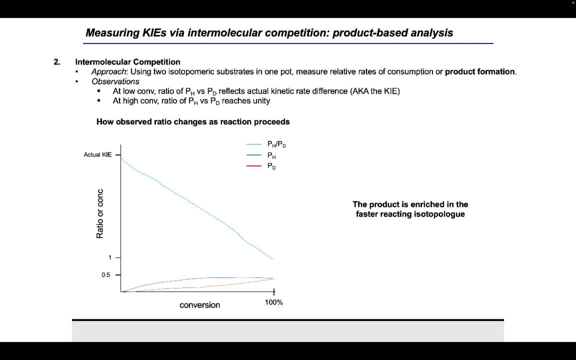 product ratio as a function of conversion. in an intermolecular competition experiment We can see that the product ratio is close to 5 at early time points, but drops off pretty drastically in the long term when the KIE is is less than a 2.4.. In this example we can 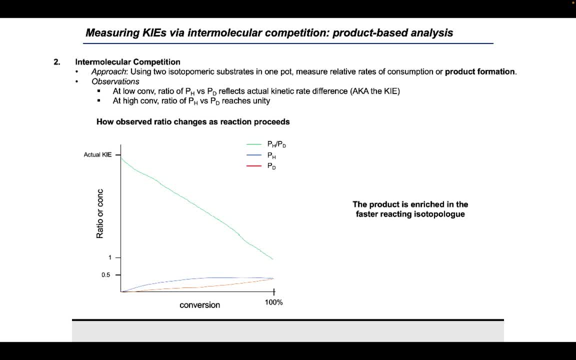 see that the KIE is does cause a significant increase in the KIE. If we take a look at the at later time points, pH is formed more quickly than PD. in this molecule The starting material H is consumed. The concentration of the starting material H. 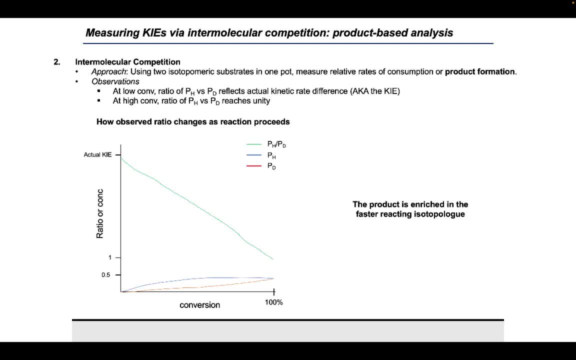 decreases relative to the starting material D. Eventually, the deuterated starting material will be in such excess to the proteated starting material that the observed rate of deuteroproduct formation will be similar to the rate of protoproduct formation, decreasing the ratio of pH-PD until it reaches unity or 1.. 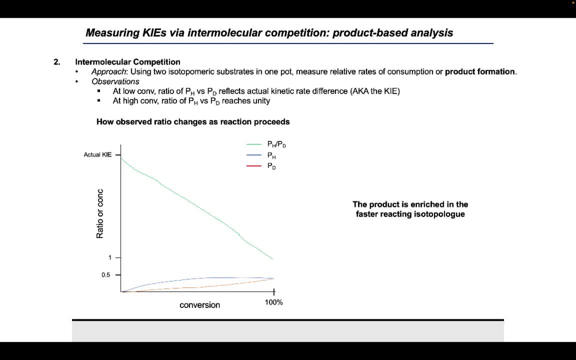 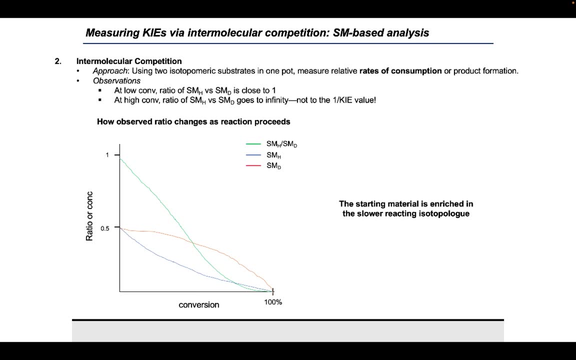 So, as you can see, that's when performing an intermolecular KIE experiment, The product ratio is only reflective of the KIE if the reaction is stopped and analyzed at early time points, aka low conversion. Now, if we switch to a starting material-based analysis, 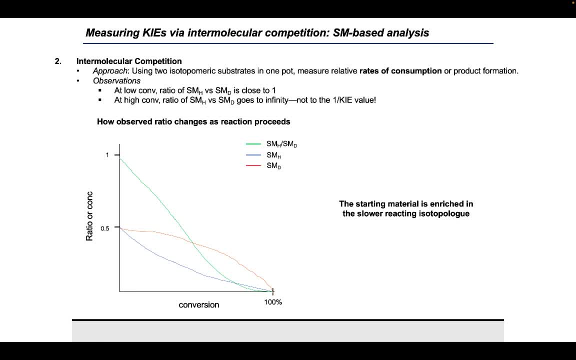 rather than a starting material-based analysis, rather than a product-based comparison of the enrichment. we see that if we start with a one-to-one mixture of the two isotopologs, this green line is constantly changing over the course of the reaction, as the more reactive isotopolog is consumed. 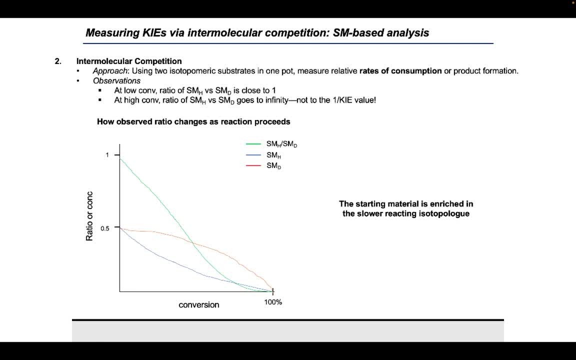 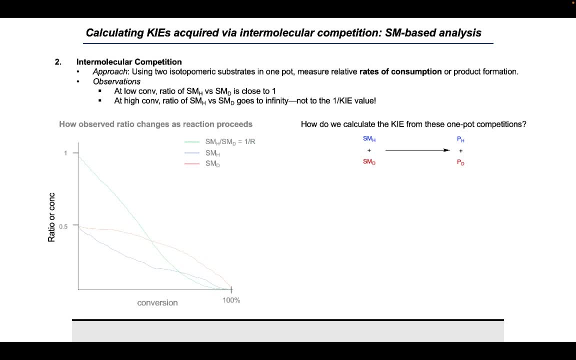 As you can see, the ratios are at their most extreme when the reaction is latest, so very high conversion. To actually determine the KIE, we need to measure the ratio of starting material or product at a specific conversion. These measurements can then be plugged into this equation. 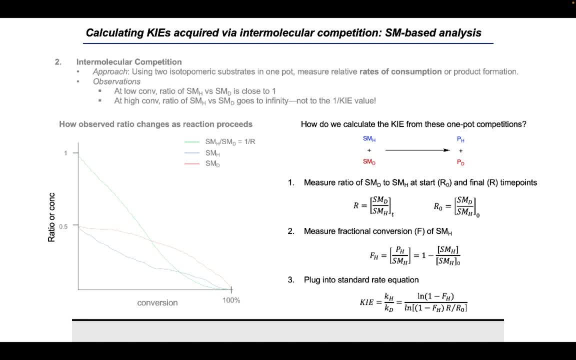 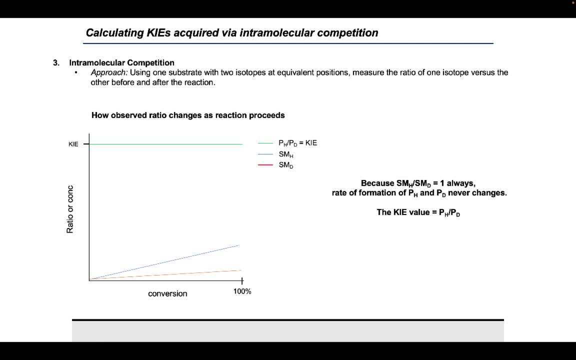 popularized by Dan Singleton, where R is the ratios and F is the fractional conversion at a given time. point Now revisiting the intramolecular competition experiment. because every molecule has one H and one D, the ratio of H to D is constant throughout the reaction. 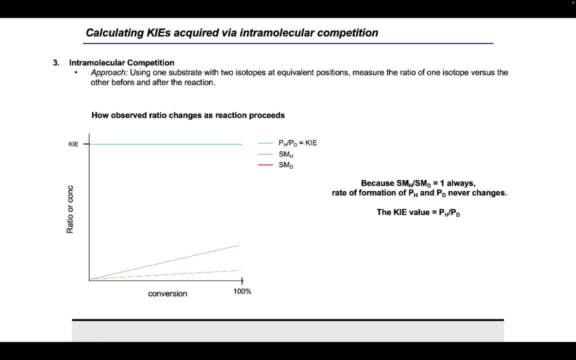 That means that the product ratio throughout any point is a faithful readout of the KIE, and so we don't have to worry about quenching the reaction and measuring conversion. Alright, before I move on to examples, I'll put up this slide again that summarizes the three ways. 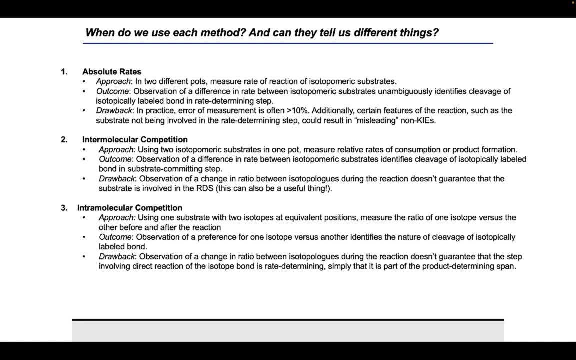 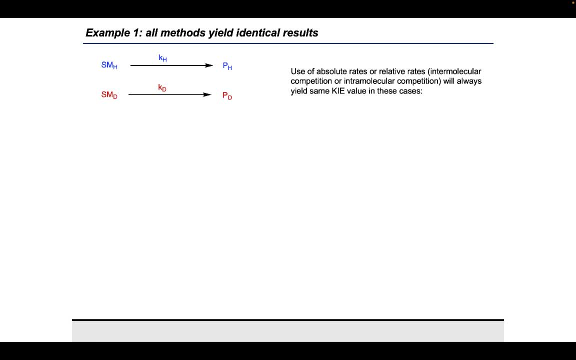 that we measure KIEs, just so that you can pause and take notes, if you'd like. Alright, let's consider some hypothetical examples and think about what we would expect from these different experiments. Now, there are many reactions where all methods will yield identical results. 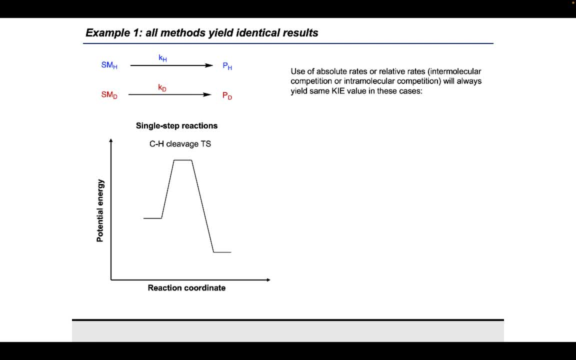 such as single-step reactions shown with this reaction coordinate on the left or, in this very specific multi-step reaction on the right, where the first step involves the highest energy transition state and is also the step that involves CH cleavage In this latter case. 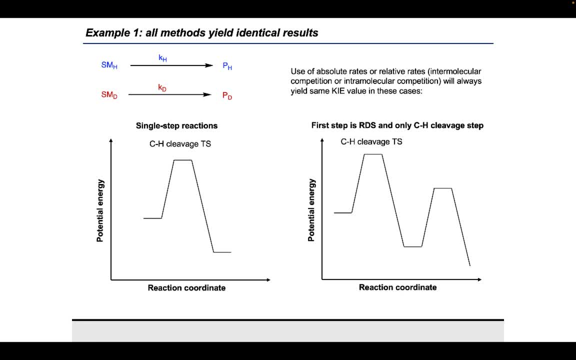 since there's just one step involving this CH bond and this is the highest kinetic barrier in the reaction, we would expect to see a KIE by all methods: absolute rates, intermolecular and intramolecular competition In this next example. 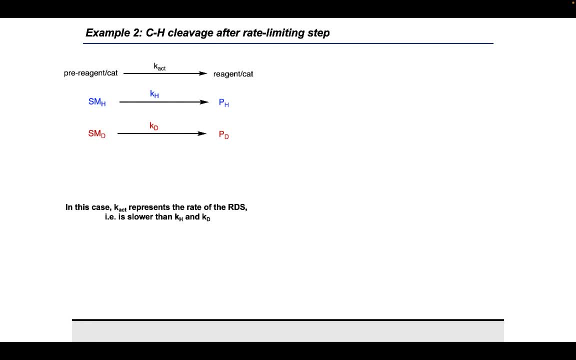 you can see that the situation becomes more complicated if CH cleavage is post-rate determining, so after the highest kinetic barrier. Now, in this scenario, the first step is rate determining. it does not involve the substrate, so thus CH cleavage occurs post-rate determining. 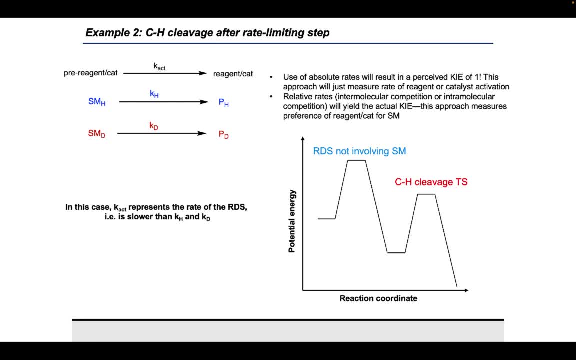 Because the rate is controlled by a step that does not involve the substrate. we will not observe a KIE from an absolute rate experiment In this example, here the rate determining step is generation of an active catalyst or reagent. However, if the rate of reaction with the catalyst or reagent 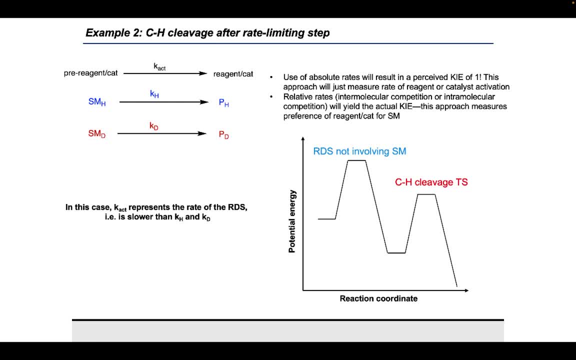 is different still. between the two isotopologs we will see an inter- and intramolecular KIE, That is, if the two isotopologs are in the same pot and if the catalyst has a preference for reacting with one isotopolog. 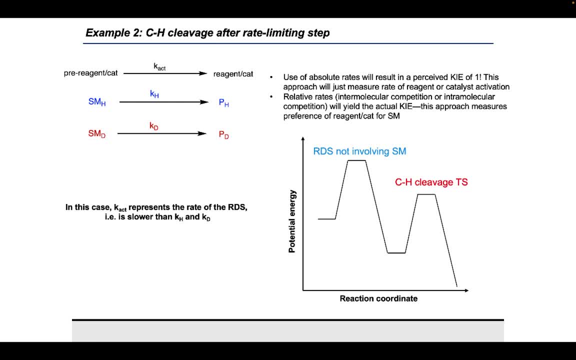 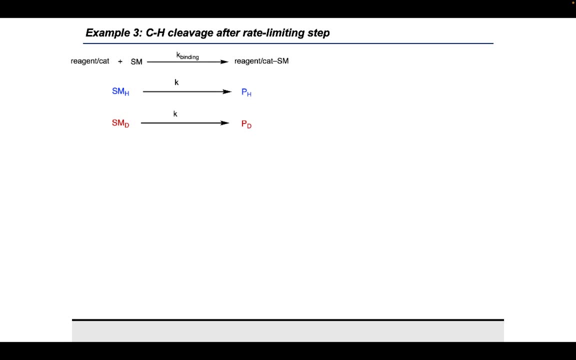 over the other. even after the rate determining step we will see a KIE by these competition experiments. So what this illustrates is the point that competition KIEs do not have to reflect the KIE of the rate determining step. Now in a third, different case. 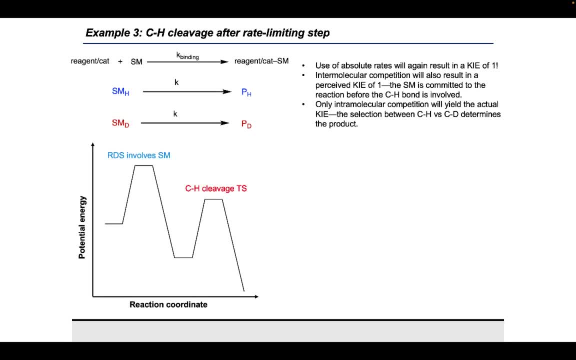 what if the rate determining step involves the substrate but does not involve CH cleavage? Examples of this could be pi-complexation to the catalyst, oxidative addition to a C-X bond, etc. Now, based on what we've already discussed, 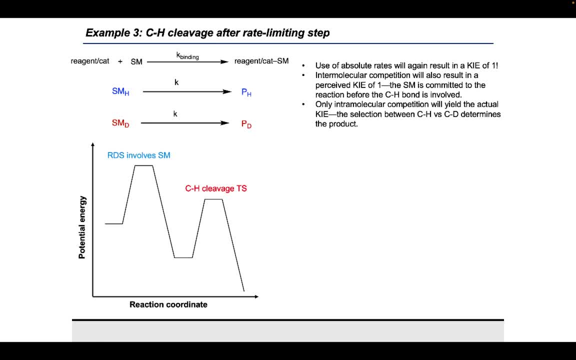 we won't see a primary KIE by absolute rates, because the CH cleavage does not happen in this rate determining step. Additionally, we would expect to see no intermolecular KIE. Let me explain. Because the catalyst binds the substrate, for example. 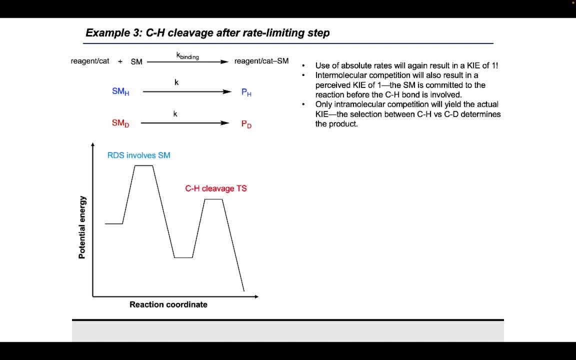 in the rate determining step, the catalyst commits to the substrate without regard for the isotope. Both isotopomers then undergo reaction at the same overall rate. The only KIE measurement we'll observe is one acquired via intramolecular competition, because the catalyst can still choose. 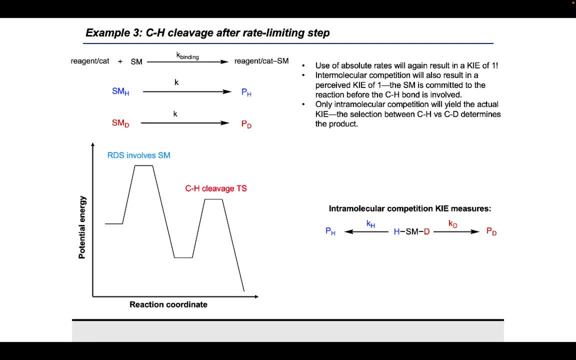 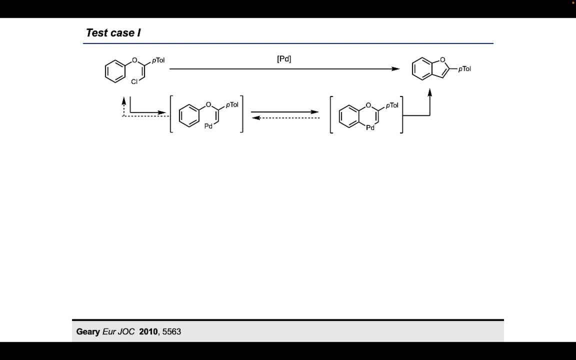 between the H and D within the substrate, even if the substrate is already bound to the catalyst. Consider now, next, this example of a palladium catalyzed reaction. Now simplifying this reaction for the sake of our analysis, there are three steps. 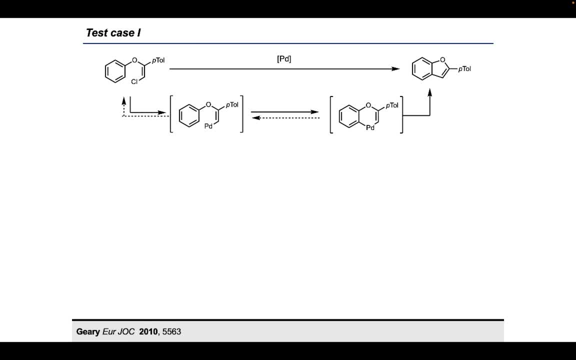 Oxidative addition, CH insertion and reductive elimination. Think about it. How can we use KIE experiments to discern which step is rate determining? With an intermolecular KIE experiment, so in the same pot, competing a substrate with a perdeuterated aryl group? 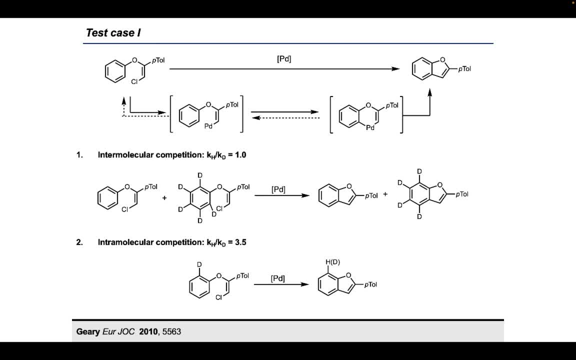 versus a substrate with a standard proteo aryl group, a lack of a KIE is observed. In contrast, use of a single substrate with one ortho-CH and one ortho-CD results in an observed KIE of 3.5.. 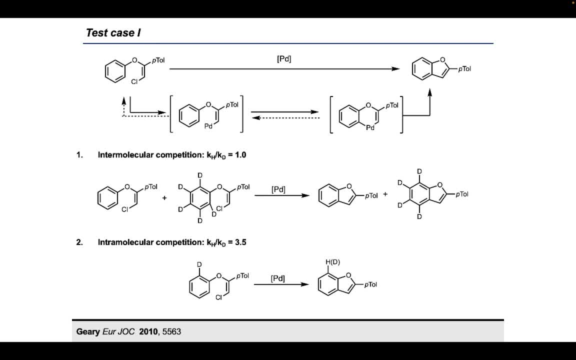 The absence of a KIE by the first intermolecular competition tells us that CH cleavage is not rate determining and that the catalyst commits to the substrate prior to the CH cleavage step. The observation of a KIE from intramolecular competition tells us that the catalyst is able to choose. 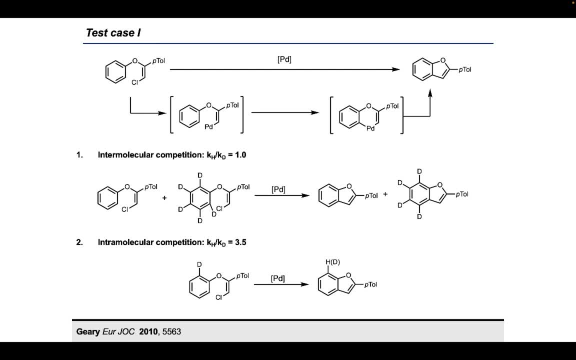 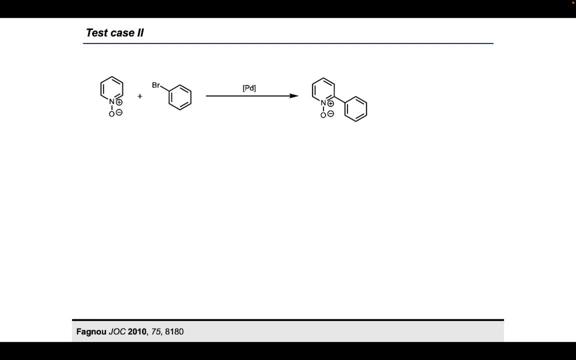 between the H and D ie selectivity is not established prior to CH cleavage. In this second example, involving a palladium-catalyzed CH arylation of a pyridine in oxide, a large KIE is observed from absolute rates. 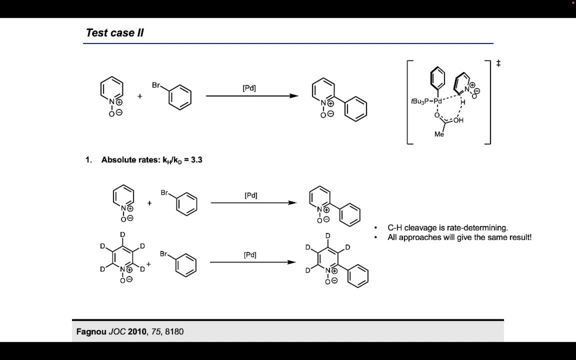 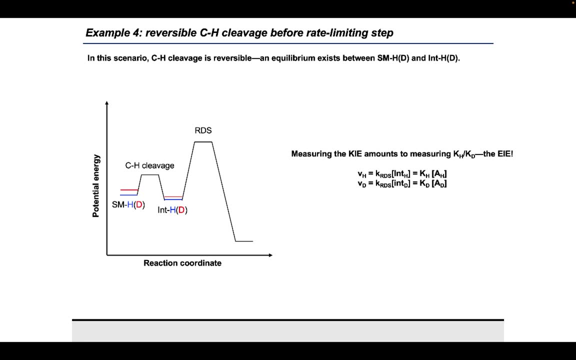 This KIE provides unambiguous evidence that the CH cleavage is rate determining, as displayed in this proposed transition state to the right. Alright, back to hypotheticals. Let's consider a fourth scenario where CH cleavage is not the first intermolecular competition. 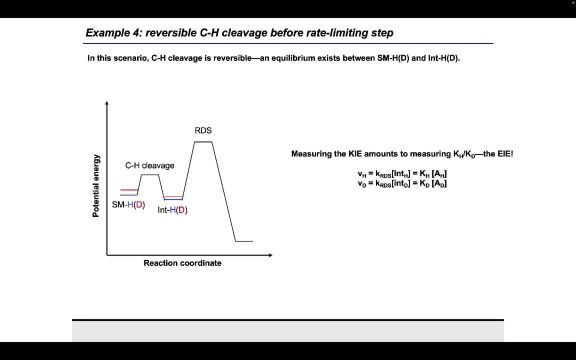 and the CH cleavage occurs prior to the rate determining step. What would we expect in this case? This actually brings us all the way back to the first part of the first section of the KIE lecture on EIEs, In this case, a measurement of the KIE. 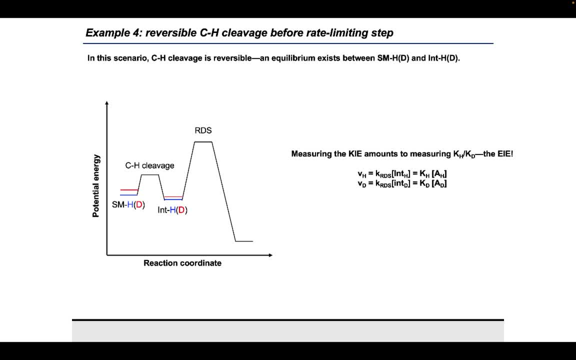 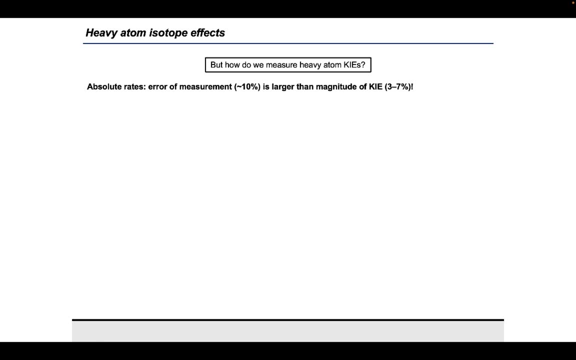 for such a reaction would amount to a measurement of the EIE for the first step of the reaction. This is because the EIE determines how much intermediate is available to undergo the rate determining step. So far, we've talked almost exclusively about HD KIEs. 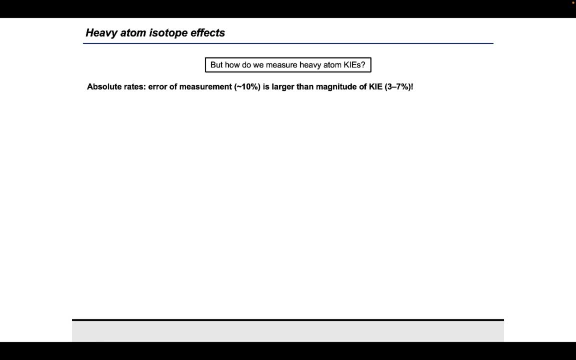 This is partially because they're useful and often straightforward to interpret. but heavy atom KIEs are also integral for mechanistic analysis. Heavy atom KIEs are much smaller because the change in reduced mass is very small compared to HD, A typical primary KIE. 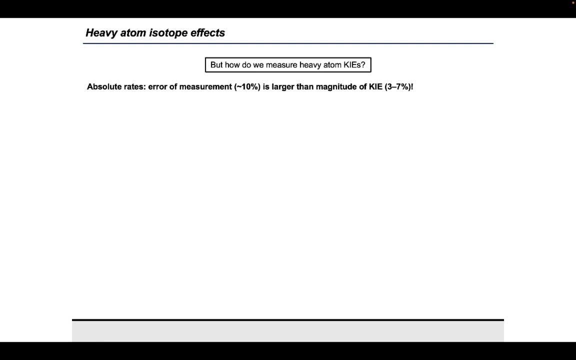 at carbon, for example, is 1.02 to 1.07.. The consequence of these small values is that it becomes virtually impossible to measure a C13 KIE by absolute rates, as measurement of absolute rates is generally prone to errors of around 5-10%. 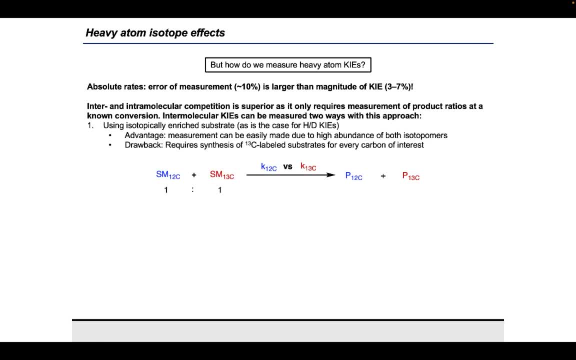 The only practical method, then, for measuring heavy atom KIEs is by either inter- or intra-molecular competition experiments. In the inter-molecular experiment, the reaction can either be taken to low conversion, where an accurate measurement of the product ratios 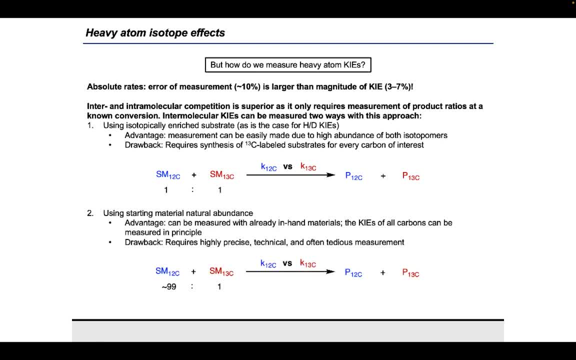 or the reaction can be taken to high conversion and then the KIE can be measured from the starting material isotopologue ratio. One thing to point out here is that the ratio of isotopologues in the starting material can be anything as long as it's known. 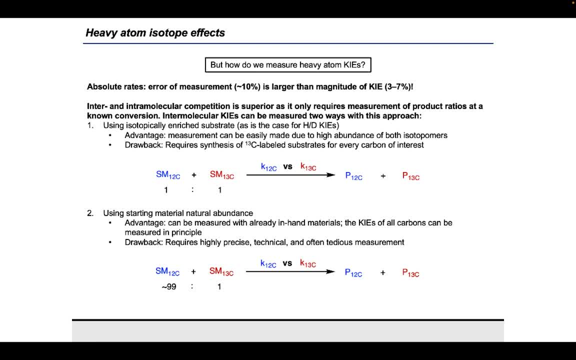 Sometimes this means intentional synthesis of C13-bearing substrates that can then be directly competed with more abundant C12-bearing substrates. However, these experiments can be done using the natural distribution of isotopes, as C13 is present at 1 out of roughly. 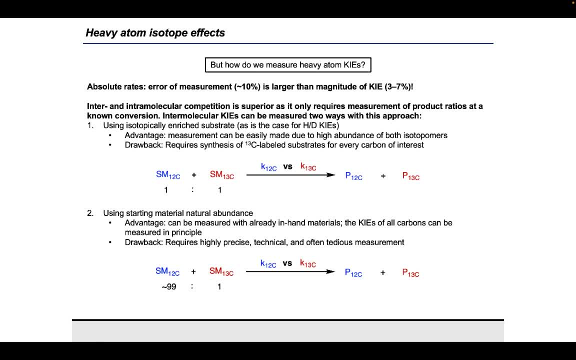 every 100 carbon atoms. This approach has the added benefit of not requiring synthesis of isotopically labeled substrates, which can be very challenging. The other benefit is that then it's possible to obtain KIE measurements at every carbon on the molecule. 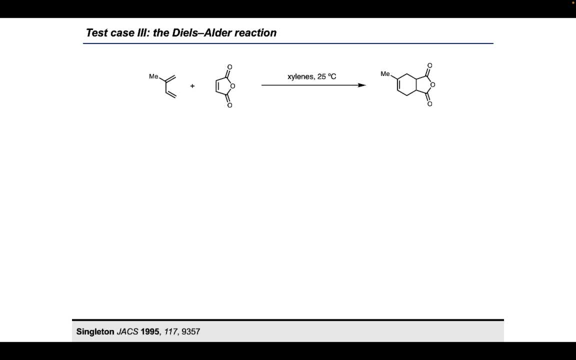 For example, let's look at this classic Diels-Alder reaction studied by Dan Singleton. In this case, the Singleton lab ran this reaction to high conversion and then measured the isotopic fractionation of the isoprene starting material. Ultimately, they were able to calculate KIEs. 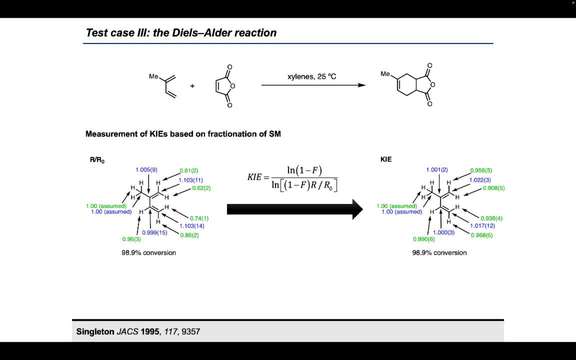 for all carbons and hydrogens. on isoprene, They observed primary KIEs at both carbons that form new bonds in the reaction, And then they also observed inverse secondary HD KIEs at the hydrogens on these carbons. since these carbons 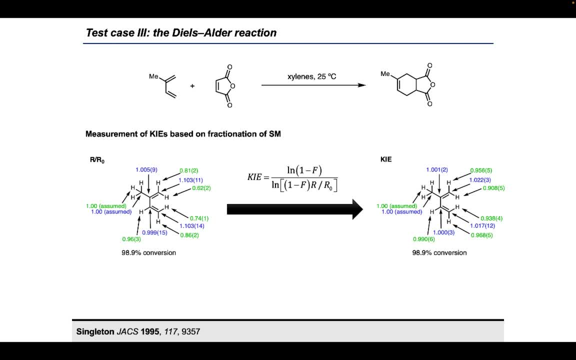 are undergoing rehybridization from sp3 to sp2.. Digging a bit further, it's notable that the two terminal carbons that undergo bond formation don't have the same KIE value. If we remember from earlier in the lecture one of the determinants of KIE values, 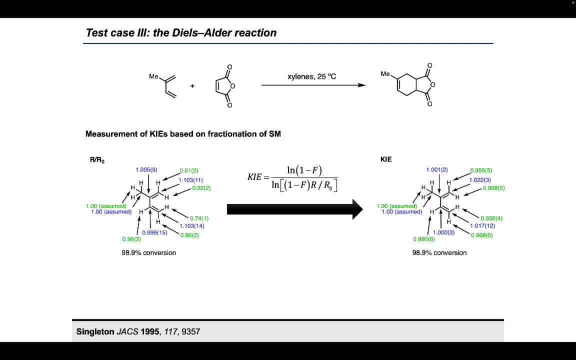 are the vibrations in the transition state, which of course arise due to the geometry in the transition state. If the KIEs are different, the bonding to these atoms must also be different. Thus, the difference in KIE values is indicative of an asynchronous 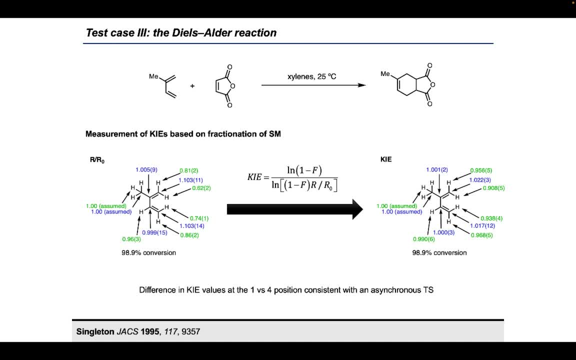 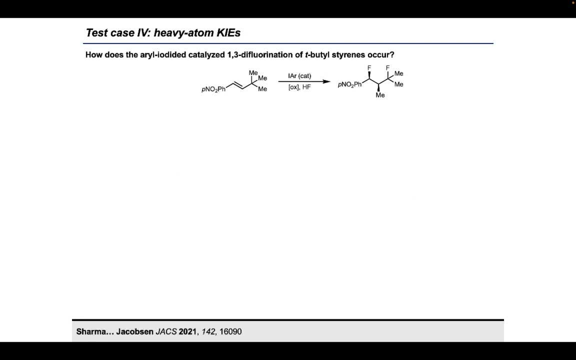 transition state. That is where the two bonds being formed are not identical. in the transition state, Let's now move on to discuss carbon KIEs in a reaction that is near and dear to my heart. Back to these 1,3-difluorination reactions. 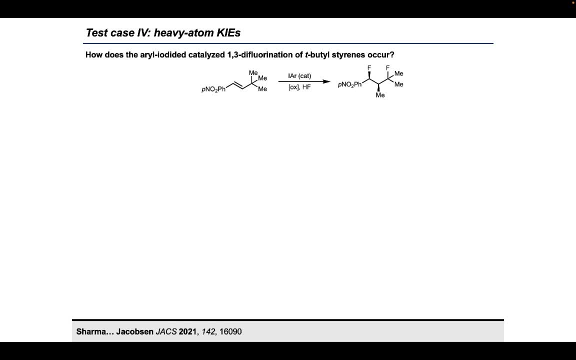 catalyzed by aryl iodide species, this time involving beta-terp-butyl styrenes rather than beta-cumyl styrenes. Now the question remains the same After aryl-iodonium complexation with the styrene. 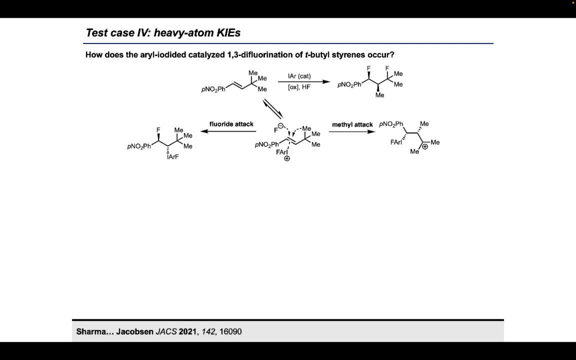 does fluoride attack first or does the methyl group migrate first? Now, if you recall, in the aryl rearrangement reaction the aryl group attacks before fluoride. We wondered if it was the same here, given that the methyl migration is much less favorable than the aryl migration. 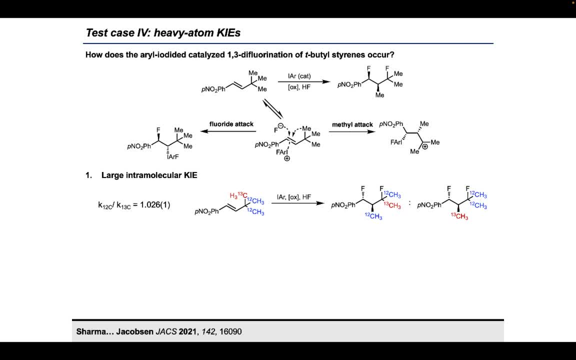 Now, in this study we used heavy atom carbon KIE experiments, which we can think of similarly to HD KIE experiments. Large KIE bond cleavage, no KIE post rate determining or substrate committing bond cleavage. When we measure the 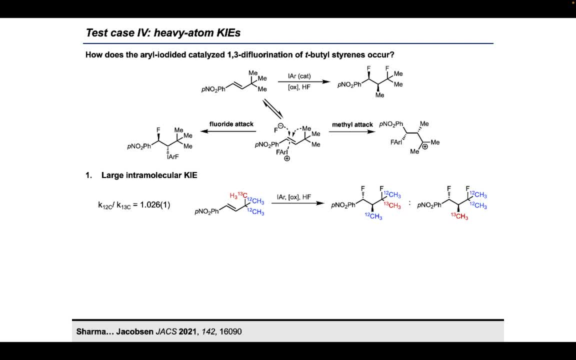 intramolecular KIE, we observe a large difference in the propensity for a carbon-13 methyl group to migrate versus a carbon-12 methyl group, resulting in a KIE of 2.6%, which, remember, is large for carbon. However, we observe 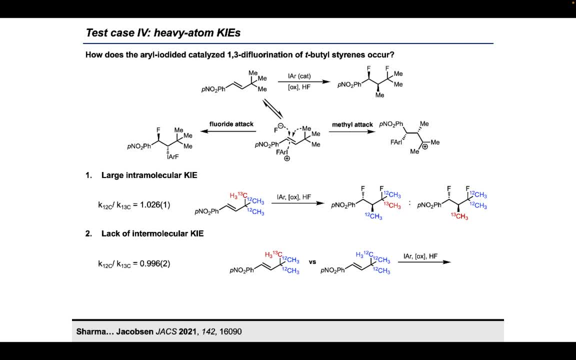 a lack of an intermolecular KIE, which is surprising because this rules out substrate committing methyl migration and is thus inconsistent with the methyl attack first pathway. Instead, this substrate reacts via fluoride, first pathway. This is the opposite of how the cumulostyrines react. 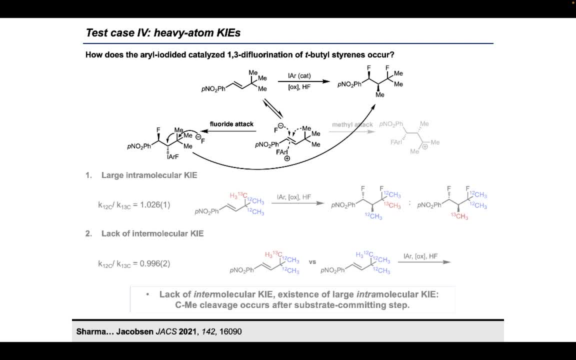 And I think this is pretty cool because it provides an example of a single reaction that can occur via different mechanisms despite featuring almost identical substrates, the same catalyst reaction conditions and very high levels of enantioselectivity for both substrates. 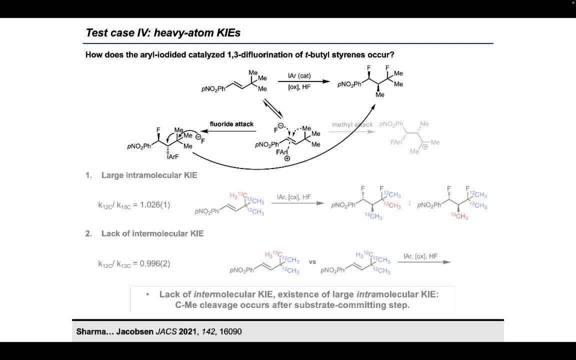 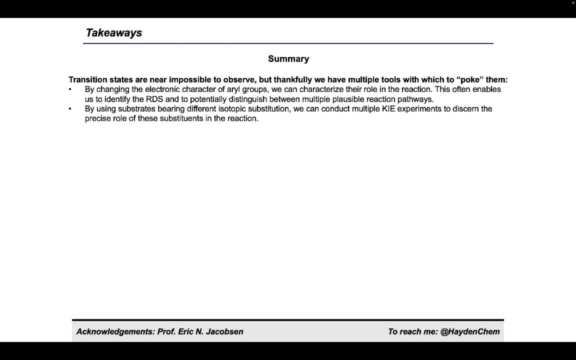 It's kind of a two for one deal. We can tease this out because of using a combination of KIE and HAMET experiments. Alright, this example ends my lecture for today. I hope that this talk has been instrumental in teaching the basis for how to design. 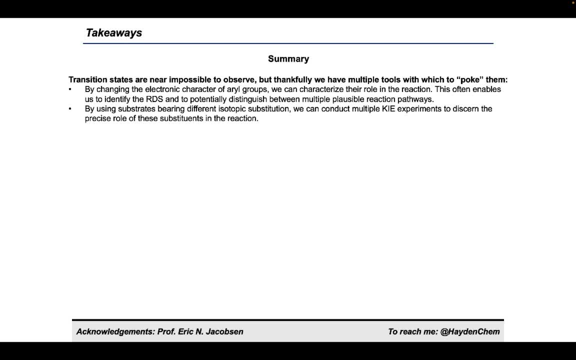 and analyze HAMET and KIE experiments, as well as giving an appreciation for the value that they bring to understanding reaction mechanisms. Really, these tools are so useful because they give us glimpses of transition states which are essentially impossible to observe directly. 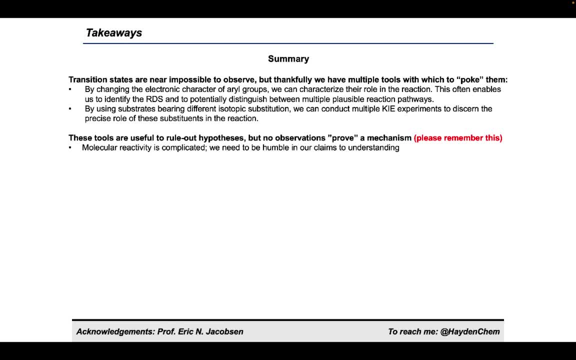 Given the rising interest in finding transition state structures using DFT, this also gives us a critical tool to validate such computational pictures, That is, if the DFT predicts some feature of the reaction that is inconsistent with HAMET or KIE studies. 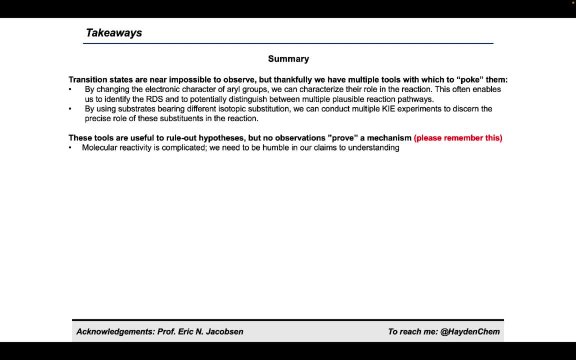 we need to reconsider the DFT. Conversely, if the DFT picture is corroborated by these studies, this gives us a lot more confidence in this picture. The second big picture takeaway slash reminder I have for you is that these tools don't prove mechanisms.